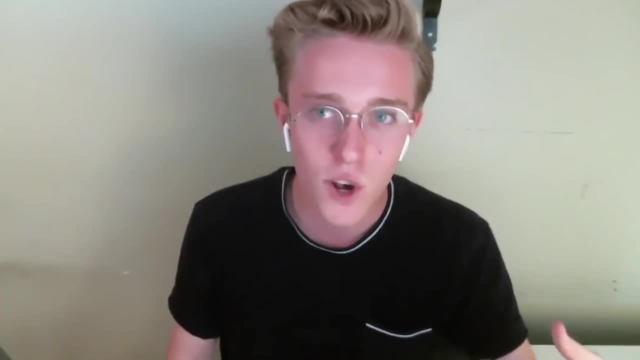 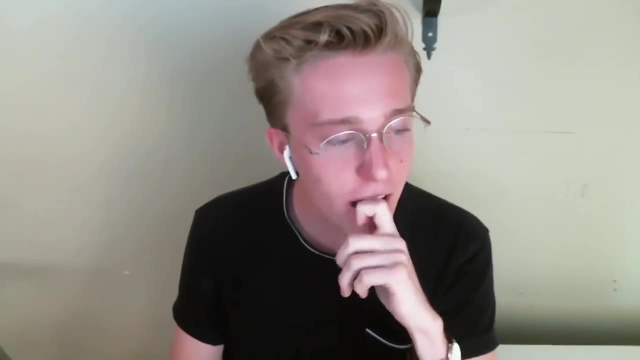 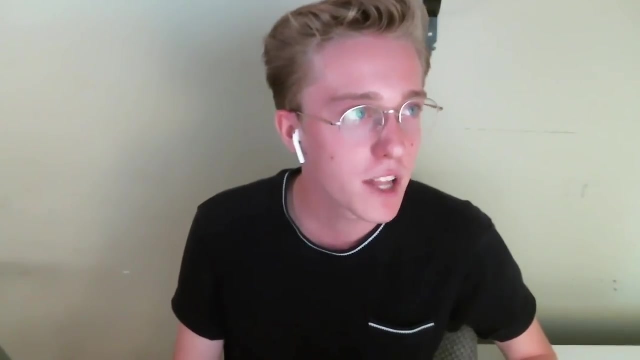 Like if I were to be charging thousands of dollars. it's just I have to know that there's something behind that to kind of justify it. I don't know. Why is that? I don't know. And the thing is, I have no problem charging. you know more, Like I understand my self-worth, but it's just I feel like other people won't see that you know. 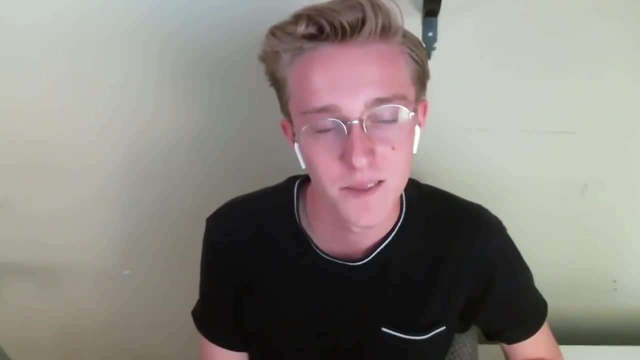 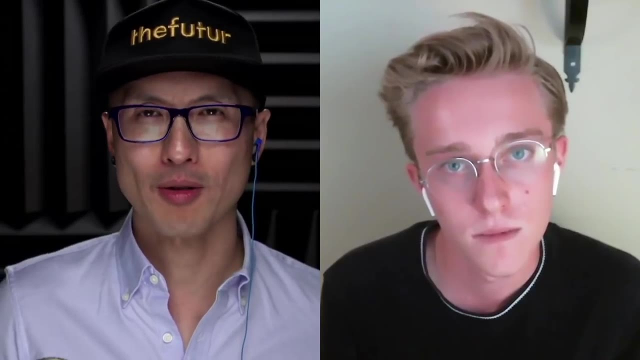 Well then, you don't understand it, because I don't care what anybody thinks or says. okay, So let's look at this: If you were to browse the internet right now and you just stumble upon a bunch of accounts on Instagram or on Behance, how do you know how old they are? 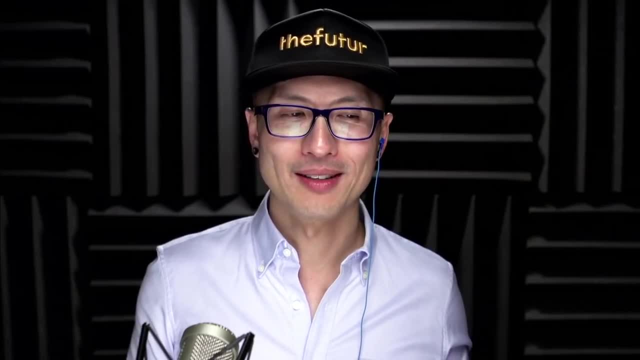 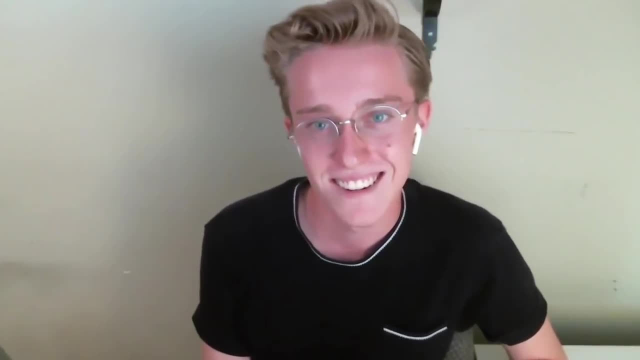 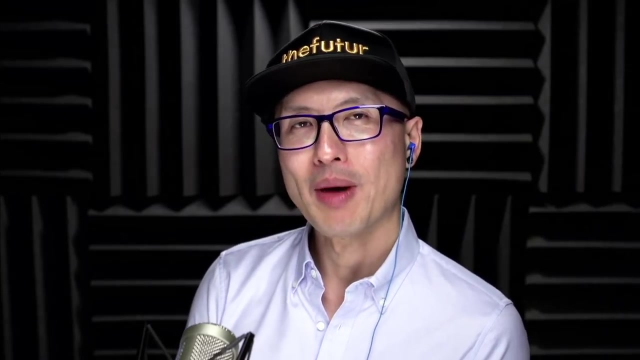 How do you know where they live? How do you know what kind of design pedigree they have? Or can you tell Spencer, I don't think you can tell directly. No, you cannot tell. I didn't get it. You can't tell period. So the answer to your question is actually easy and obvious, which is: you do good work, you put good work out there, and it doesn't matter if you're 17,, 7, or 77. 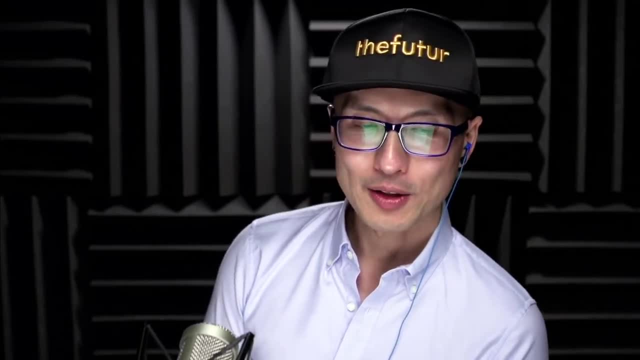 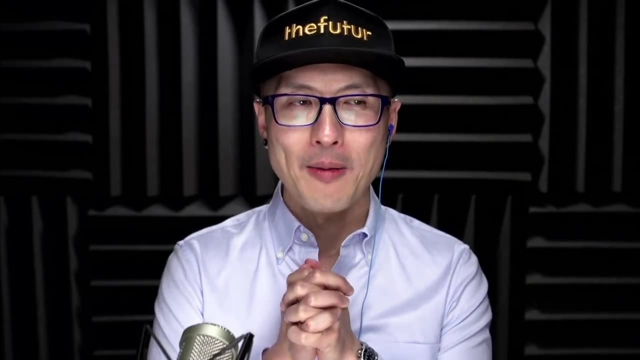 It doesn't matter at all, okay. So now let's talk about your self-worth. You say I'm worth it, but other people won't see that. That's not coming from the voice of a person who's saying that. 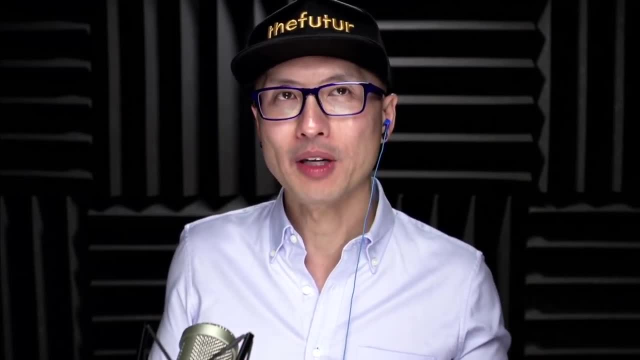 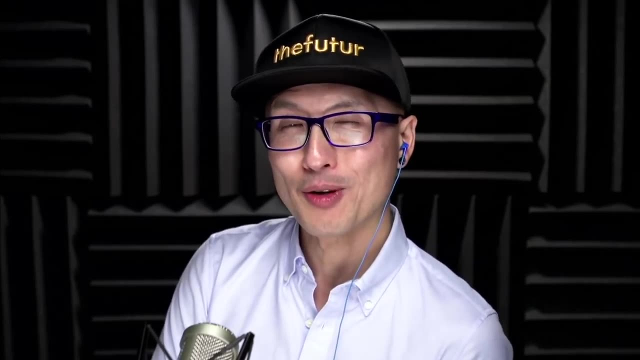 I say I'm worth it. It's too bad you can't see it, so I'll find somebody who sees the worth. That's it, Okay. Okay Now, no matter how much I charge- and you guys have heard me drop astronomical numbers compared to the numbers that you're seeing, and yet I still think it's a discount- 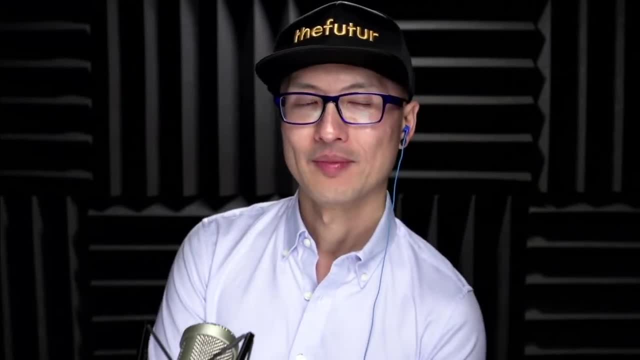 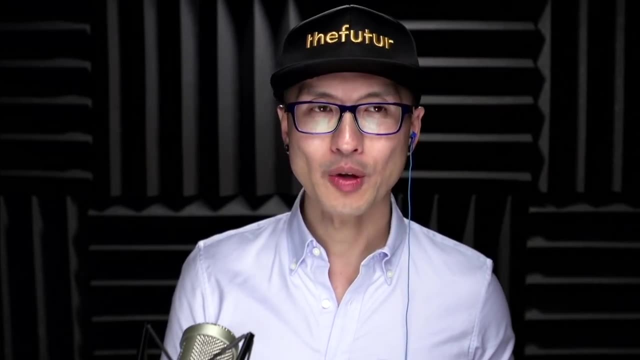 No matter how much money I charge. I think it should be higher, okay. So if you start to learn to believe in yourself- and it's okay because you're 17,, 18 years old- right now you're going to high school- you haven't yet come to your own full power and to know what you're capable of doing, 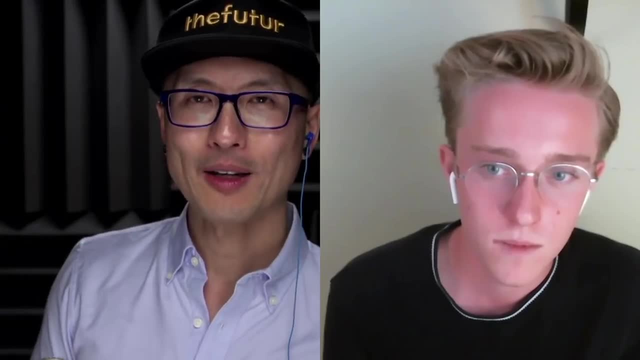 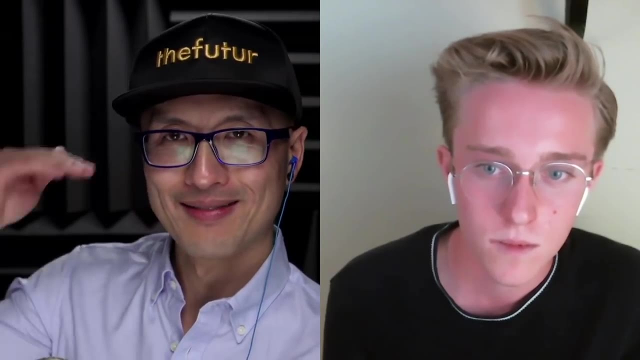 You still have things to learn. You still have things to learn in your life and that's okay. I don't want you to walk out there at 17 or 18 saying I learned a few things in my commercial art class in high school and now I'm just that's it. 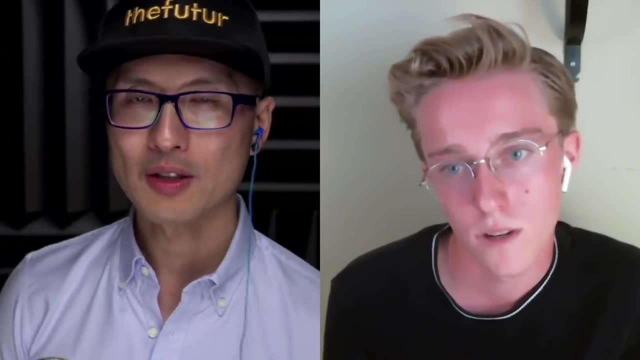 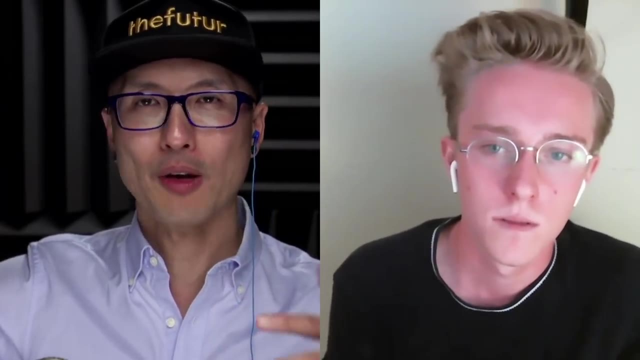 That's the highest achievement. That's as much as I need to learn. There's still a lot of things you need to learn, and just know this: There's great potential and value in you. You're just trying to align your own life experiences to meet that value that you already see in yourself. 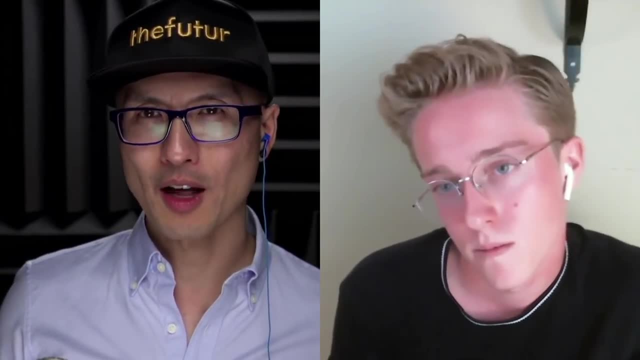 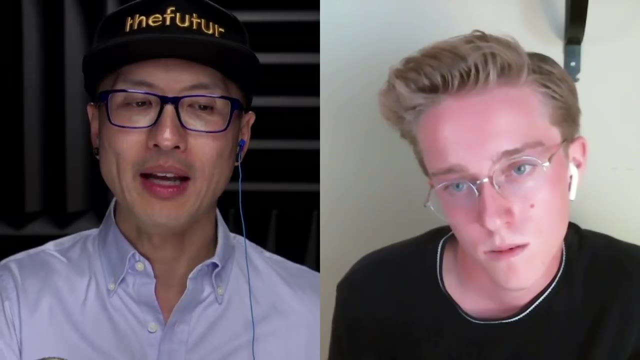 Let me say that in a different way. I want to charge a million dollars for the things that I do. I know I'm worth at least that amount of money And I'm going to keep working towards that until somebody actually sees the same value that I see in myself. 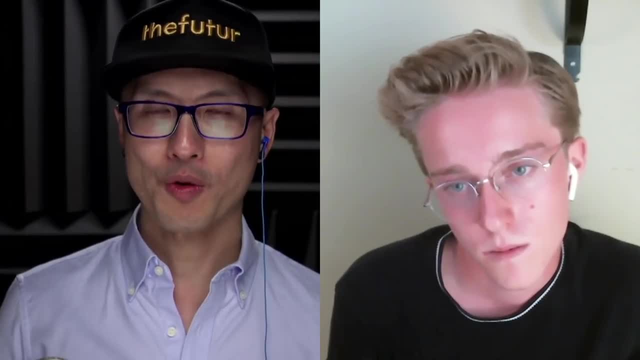 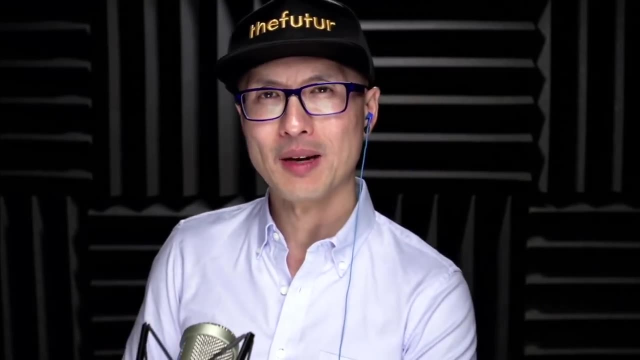 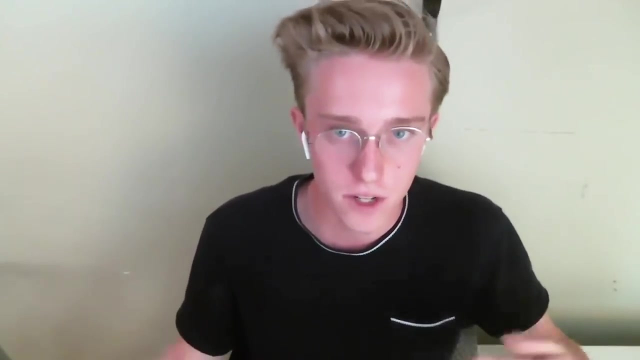 So that means I need to acquire greater skills, I need to learn more things and I need to have more experiences to help people so that they can see the same image I see of myself. So I remember from previous videos you talking about like charging on value, that kind of thing, like charging on output versus input, these kinds of things. 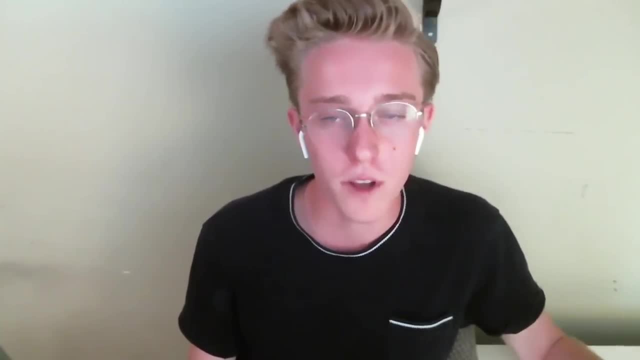 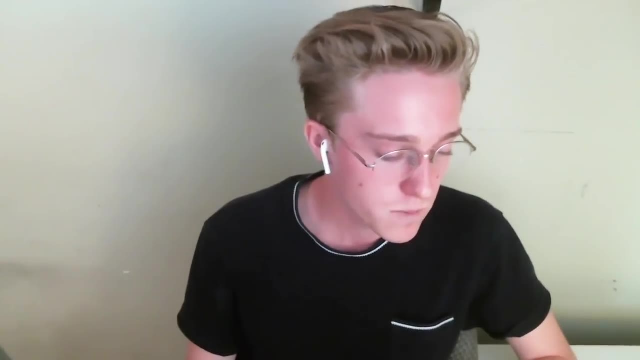 And that if you want to, you know, be more valuable, you have to solve problems other than graphic problems. Yes, Stuff like that, Yes, yes, yes, Keep going. So I remember that And I believe in that, But part of the issue is like: right now, I just solve graphic problems. 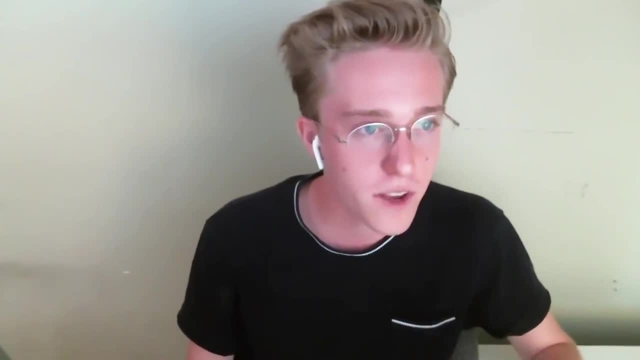 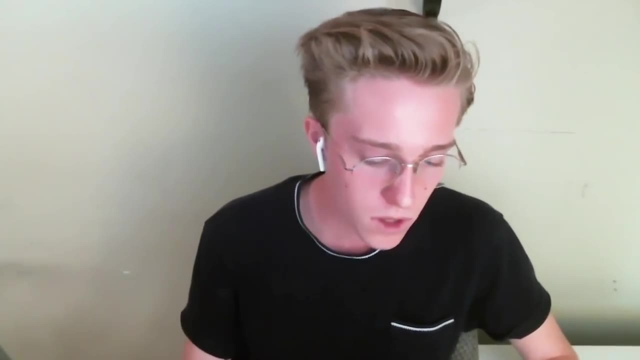 You know, Yeah, So that's part of it is just like I walk in and I know that what I do is worth money And I know that if I sat down with a client I could, you know, solve major graphic problems essentially. 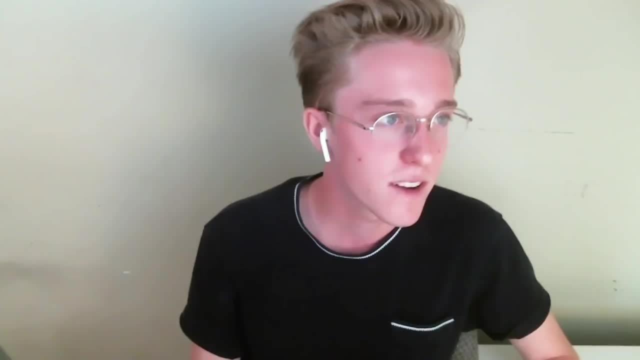 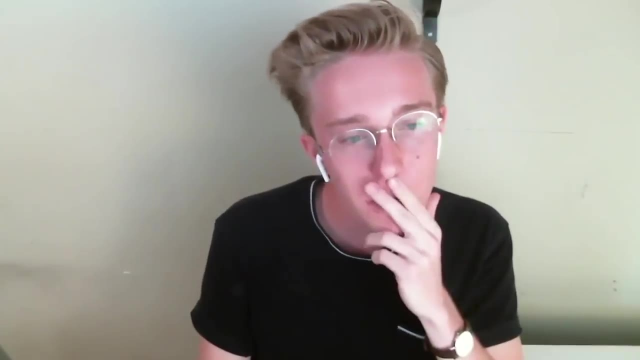 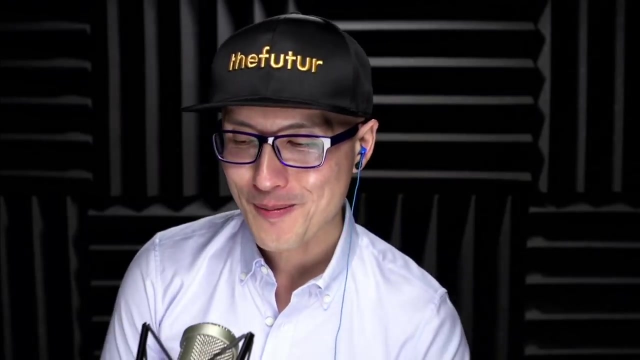 But I just, I don't know, Like is it? it's just, That's part of where the I don't know like this crossroads, I don't know. Okay, This is why sometimes now I go on stage and I say: hi, my name is Chris Doe. 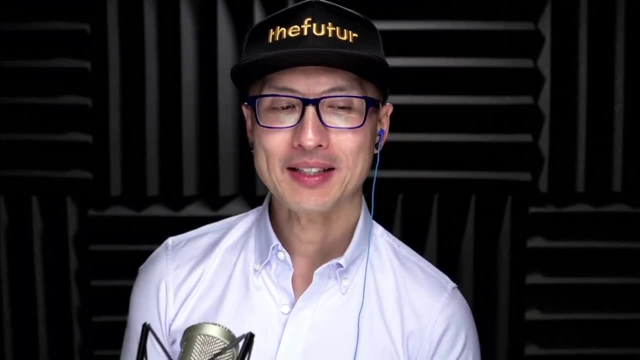 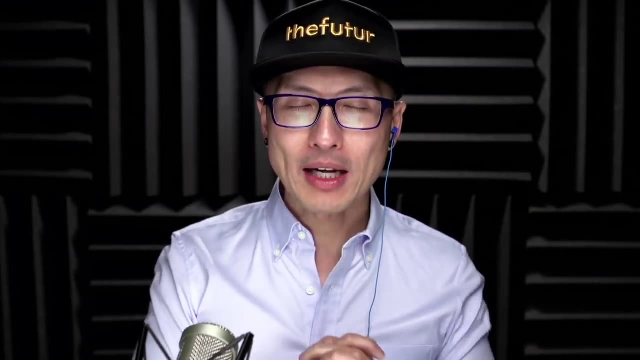 I'm a recovering graphic designer And it's because I don't want to solve graphic design problems anymore, because I'm capable of solving much bigger problems. Now some people who watch this, who are purists, who are great craftspeople, say that's heresy. 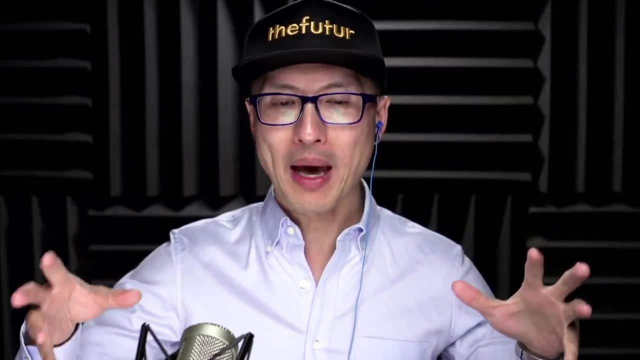 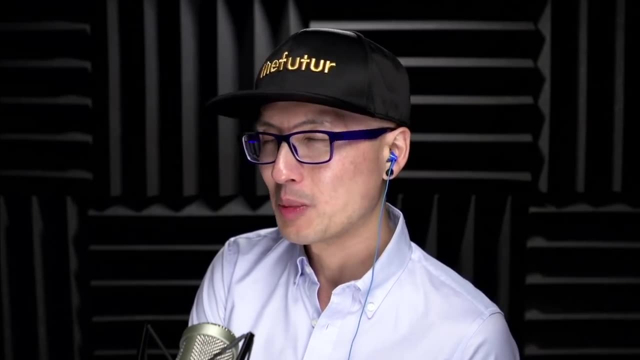 That's a bunch of BS, That's a bunch of malarkey that you're just peddling, That you're just peddling out there, And I don't think so at all. If you look at Brian Collins, he talks about them being an experienced design company. 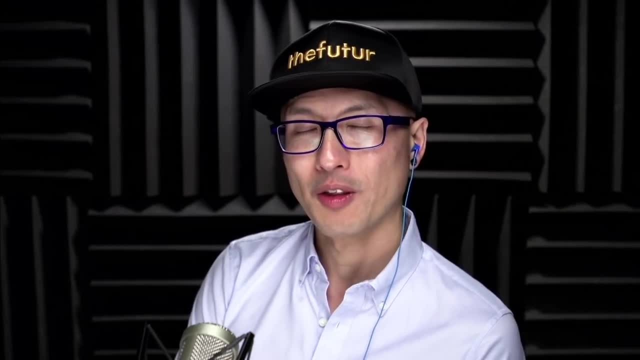 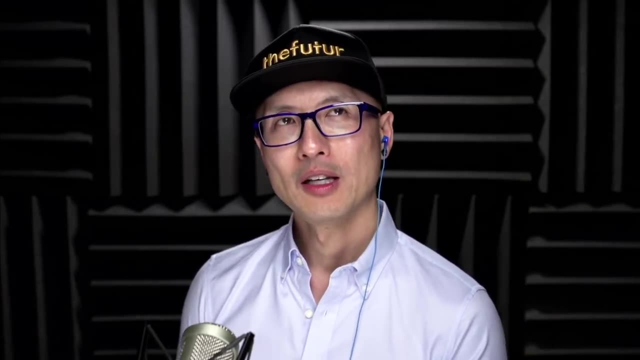 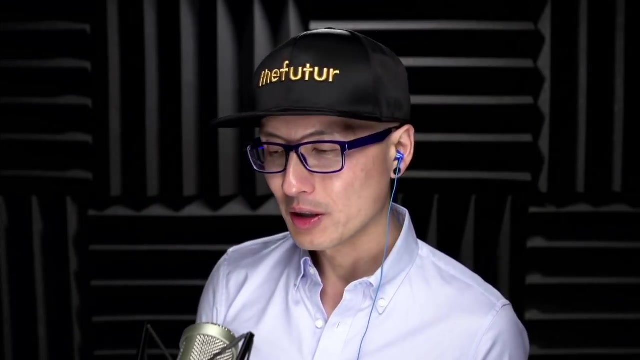 And so they're designing experiences through lots of different things, through copywriting, through image making, through user interface design. Whatever it is that they need to do, they're going to use the full extent of their creativity to solve a problem. So if a person tells me I have a conversion issue, where people are coming on the site and the bounce rate's too high, 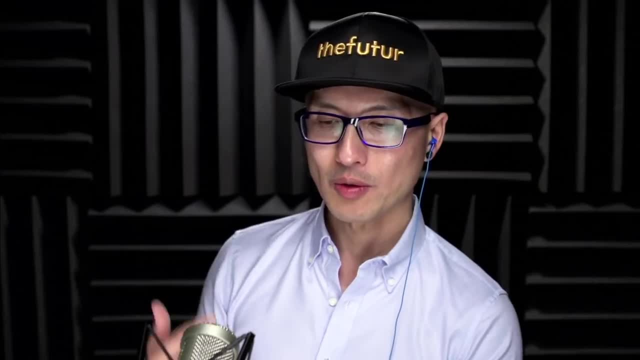 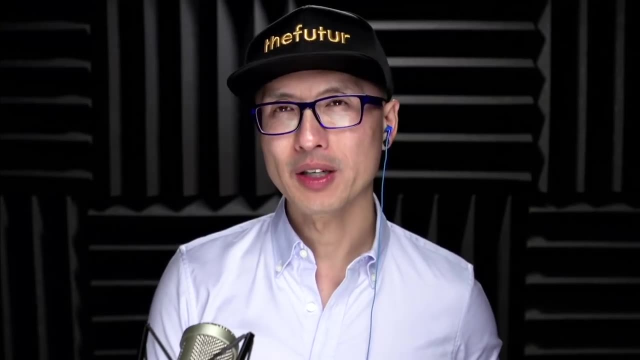 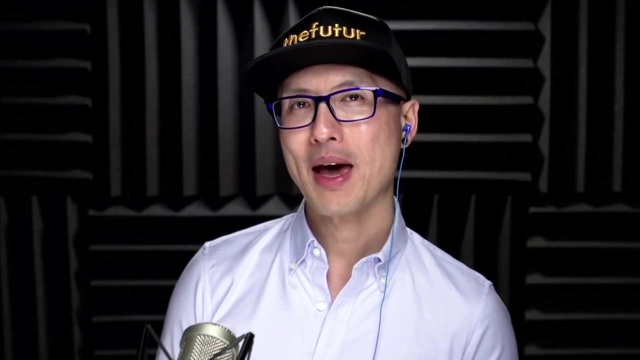 Or they're not buying as often as they should be relative to industry standards. I want to fix that problem, And sometimes that means that I have to do something that I'm not trained to do, which is most of the time. So if I come into it saying you need a new logo every single time, then it doesn't really matter what the problem is. 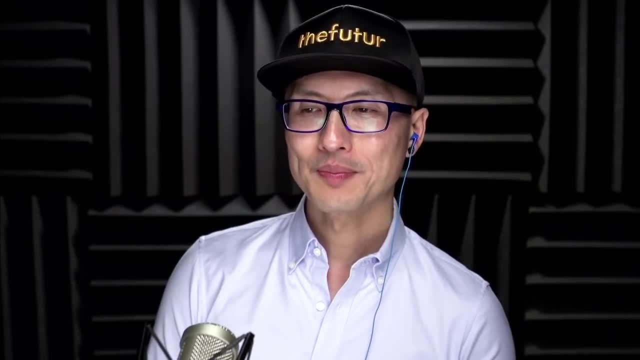 The answer cannot always be the same. right, We can understand that, right? Yeah, of course. Okay, So that's where I have to stop myself to say like, just because I love to make logos doesn't mean this person can't do it. 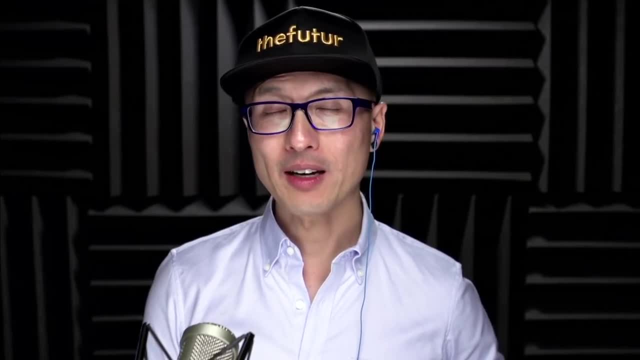 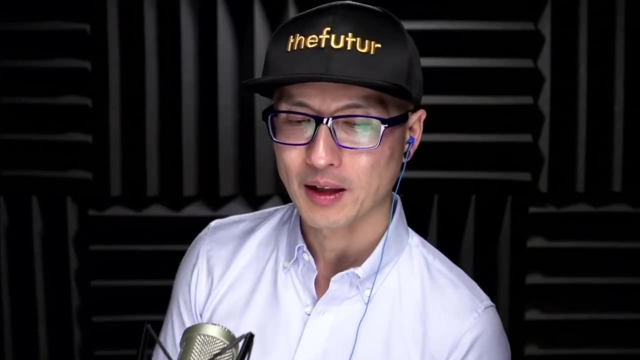 This person needs a logo. I need to kind of think about the problem and find an appropriate solution. So the best thing that you can do for yourself as a young, aspiring graphic designer- I'm speaking to you specifically, but to everybody else that's watching this- 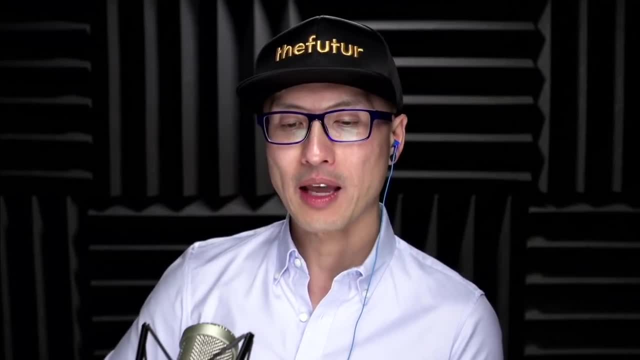 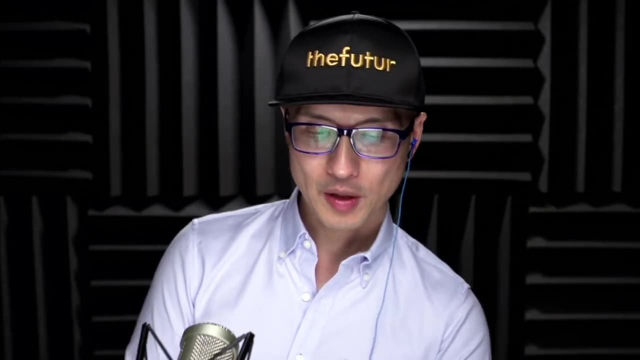 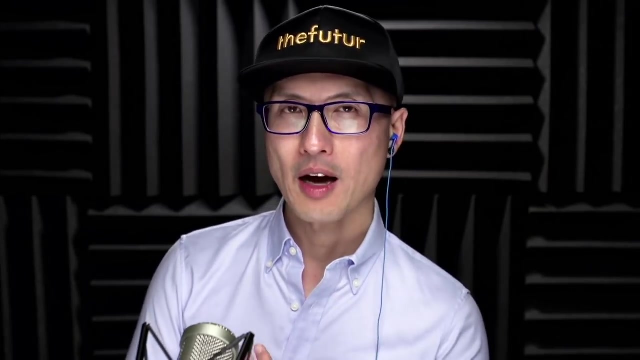 is. it's good to learn your skill and to understand foundational principles of graphic design and to have the 10,000 hours of practice that somebody like Connor has had, But then also to broaden the disciplines in which you study, Maybe to include psychology. 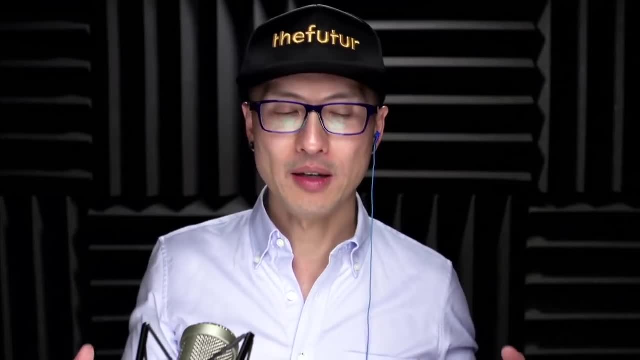 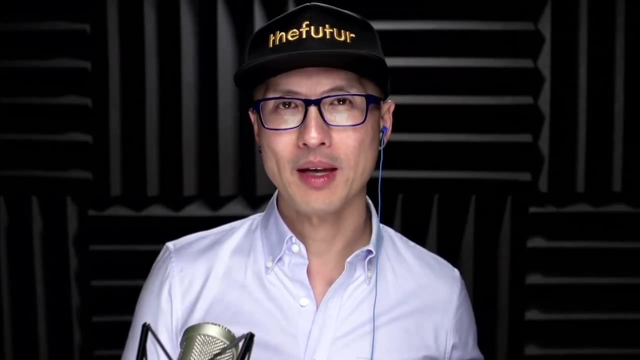 Philosophy, Anthropology- Something else to include in your mix so that, when a new problem comes, you have skill sets that go beyond just I know how to make a logo, Okay, And it sounds to me like you are exploring those things already, and I think that's good. 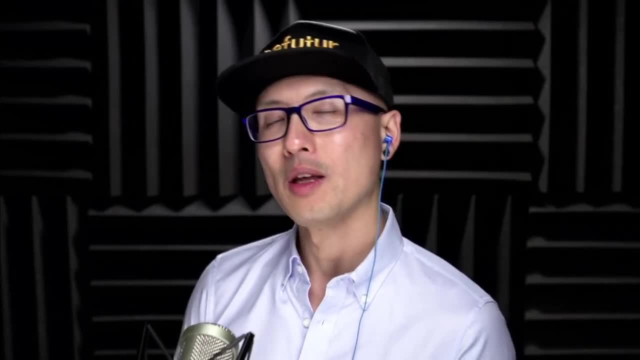 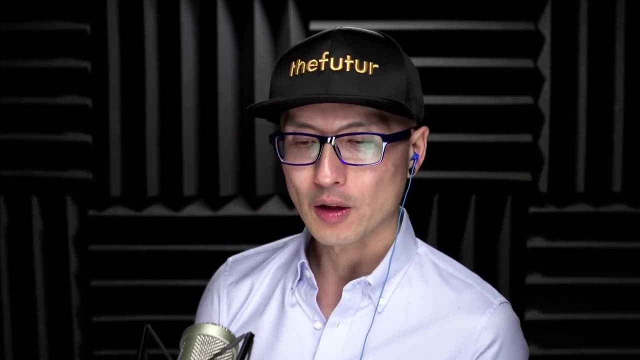 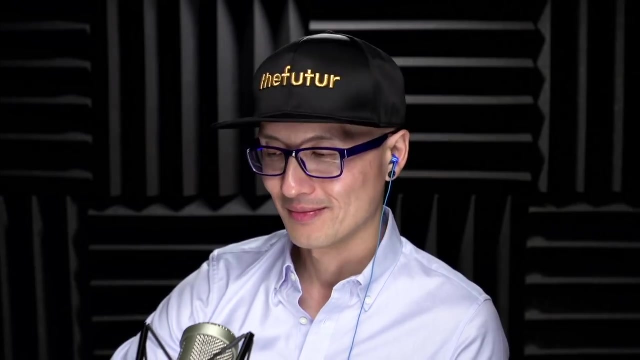 As you're about to go into college pretty soon, be open to the humanities, to literature, to mythology, to rhetoric. Those kinds of things will help you more than just learning more craftsmanship. If you're like dipping your toes in a lot of things, like you said, like explore a lot of things, 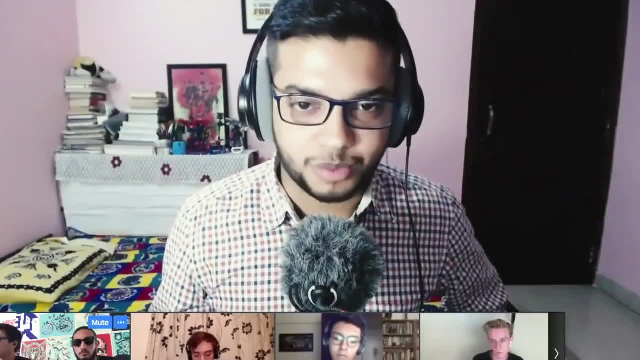 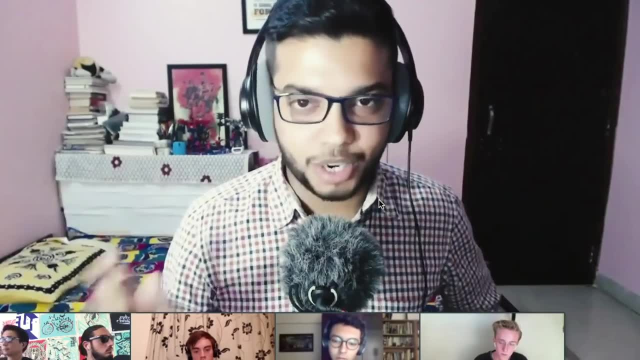 and then you get to a point where you can solve a lot of problems, right? Not just the graphic problems, Yeah. So then how do you come back from there and basically focus down to one particular thing, Like what do you get known for? 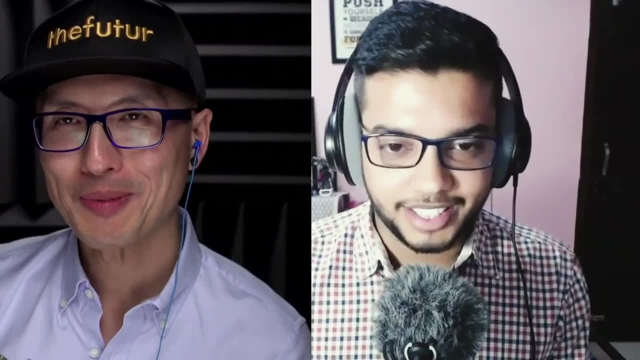 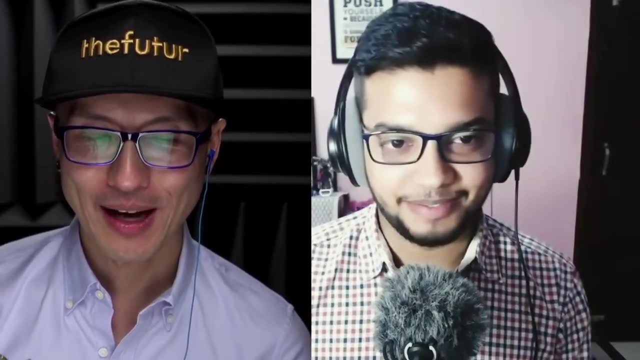 You're not an expert in one thing, right? No, I'm an expert. I'm an expert at solving problems for a lot of money. Let me ask you this question: Why are you guys talking to me right now? Why would people hire us if I am openly admitting that this is what I like to do? 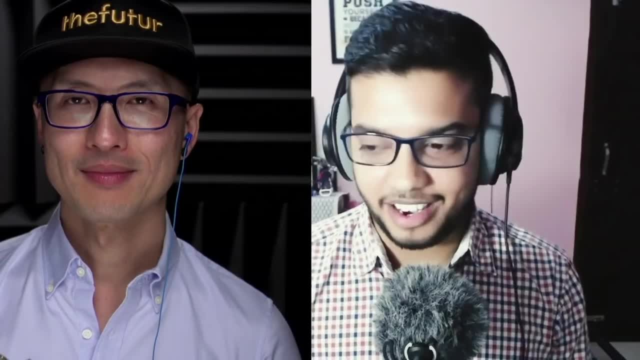 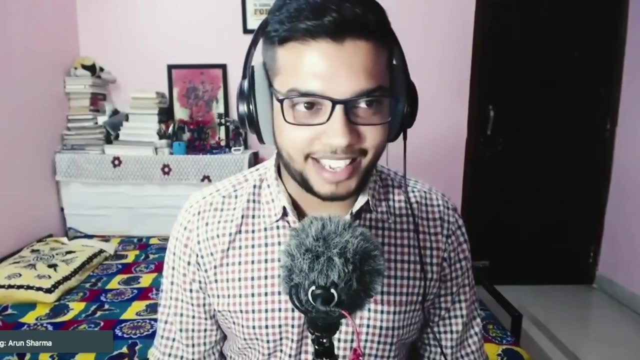 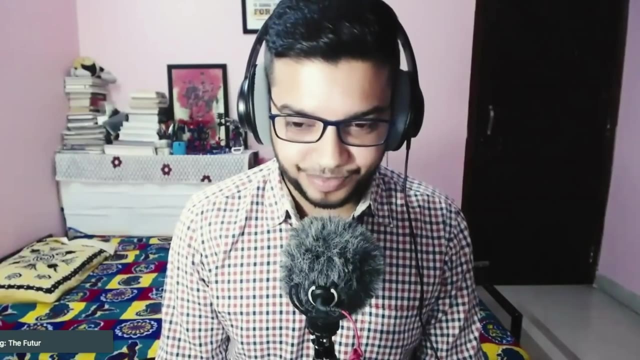 What's happening here? What do you see me as, then? You're like a teacher for, like I mean, life problems, I guess, business, career problem, Yeah, Okay, So aren't I doing exactly what I tell you to do? and do you have a problem perceiving me as an expert? 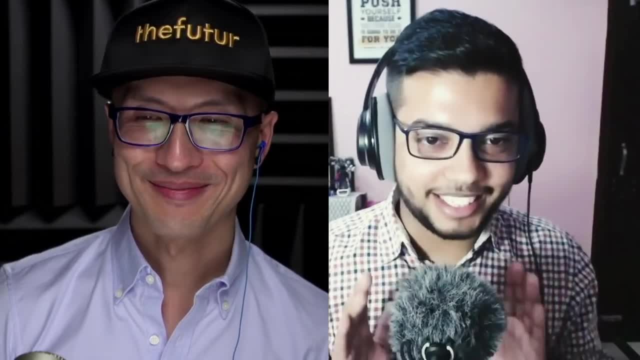 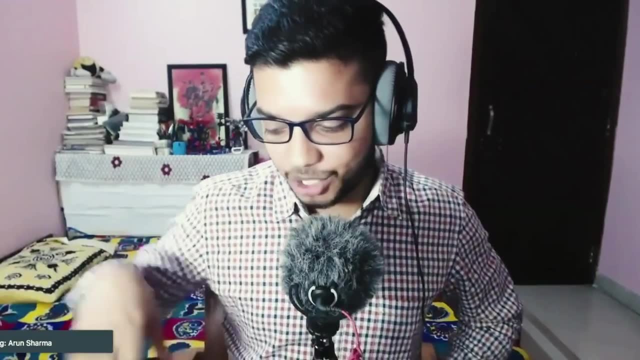 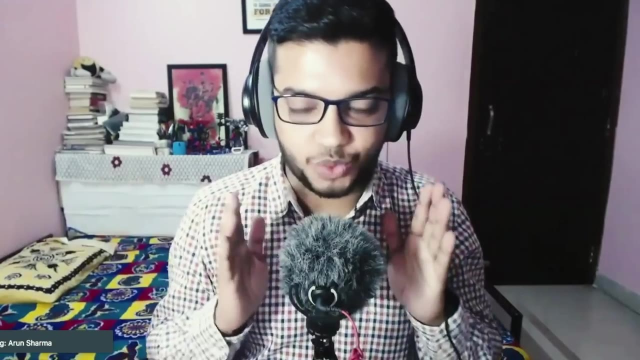 I know what you're getting to, But what I mean is: yeah, what I mean is: how do you basically tell like position yourself on, let's say, the website? Okay, you know what. like you know, this is what I do. 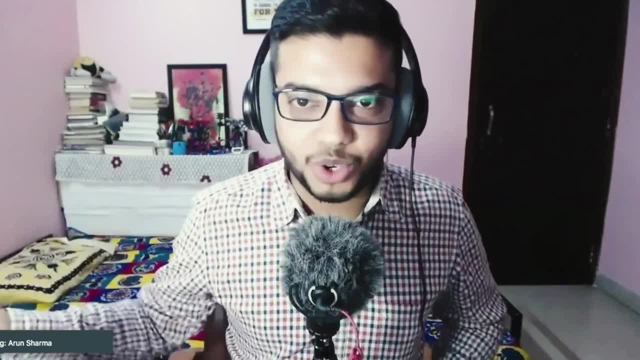 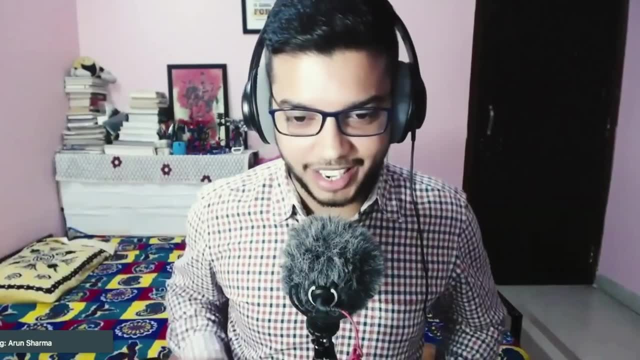 I mean, do you just say I solve problems? or like how it goes? Like Connor does just logo design, right, So he's known for just logo design. I don't just do logo design. Okay, Put him in a box, Yeah. 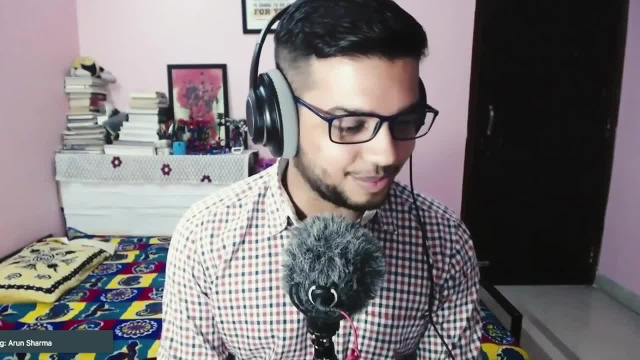 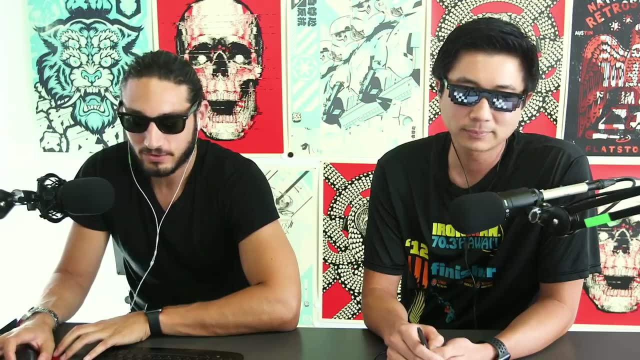 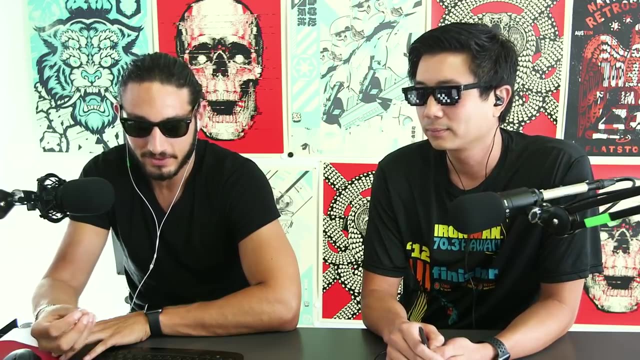 So I'm not sure if I mean, I get the question right, But I don't know. Are you asking, like, how to phrase like, if you just are a designer like you guys, all you guys, young guns, how do you phrase that on the website so that you can seem like a problem solving guy like Chris? 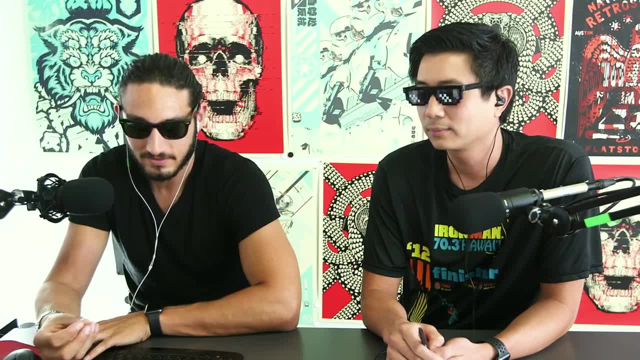 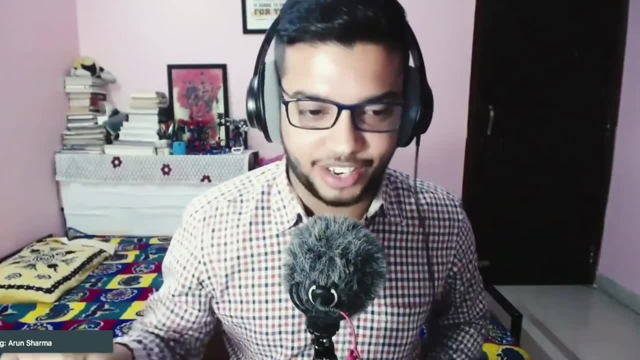 Is that what you're saying? No, I'm saying. I'm actually saying the opposite of it. Like if you're solving a lot of problems, how do you, How do you, come back and say I'm an expert at solving this kind of problem? 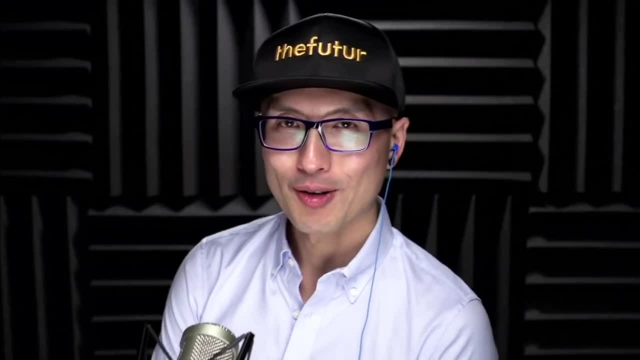 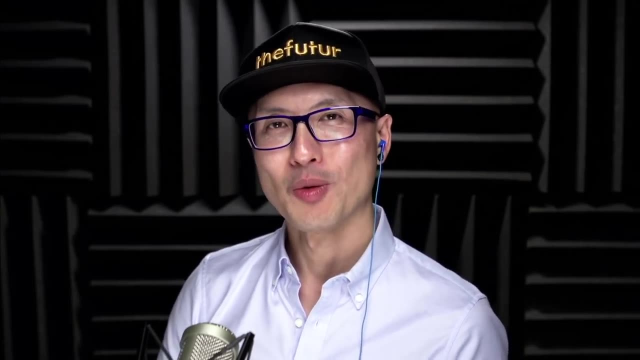 Well, why do you have to say okay, first of all, you're not in danger of saying that just today because you're not an expert at solving all kinds of problems yet, right? So we all have to start somewhere Now. remember you guys, I'm double your age right now. 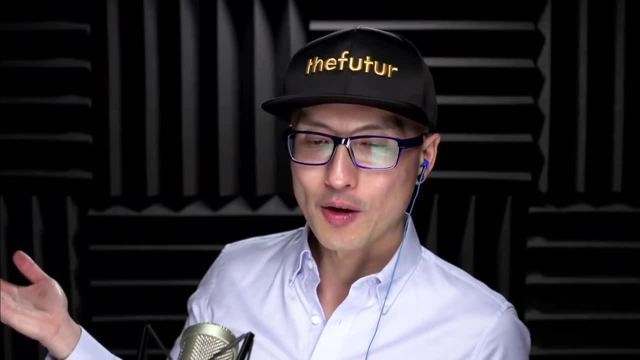 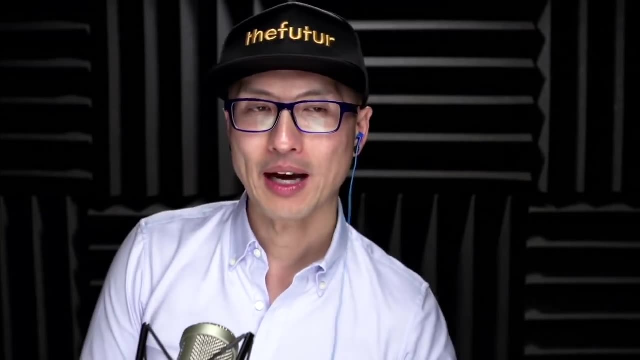 So I have a lot of experience in my life and you're trying to just make this hyper shortcut and jump to the end And you might be able to do that. Some of you might be able to. I'm not discounting that, But more often than not I can save you some time so you don't have to spend 20 years trying to figure it out. 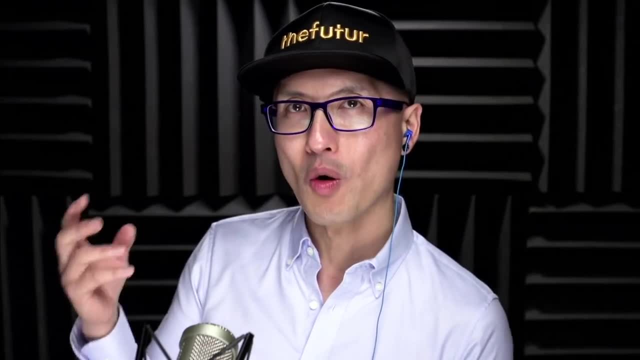 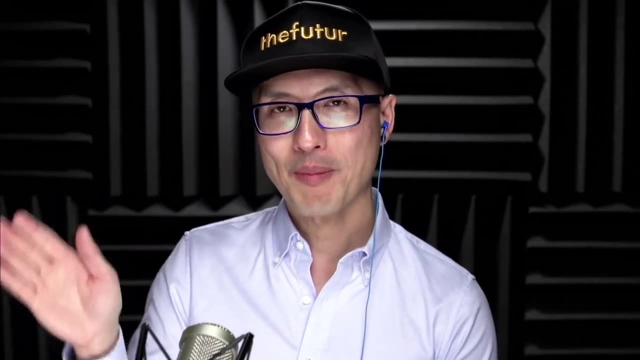 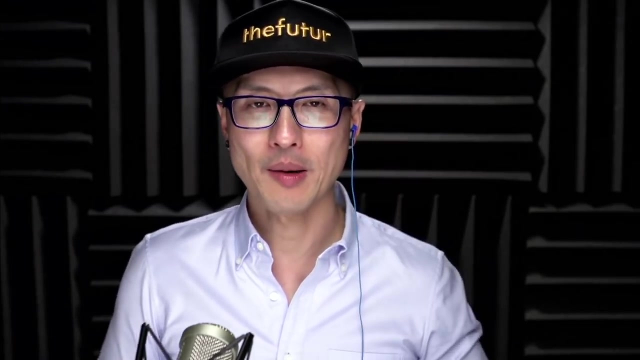 But maybe you spend six years figuring it out. So right now, if you know that your goal is to learn how to solve more complex problems that people find to be valuable, then you align your life towards that path And you read books, you go to seminars, you watch videos, you take courses that help you understand that a little bit better. 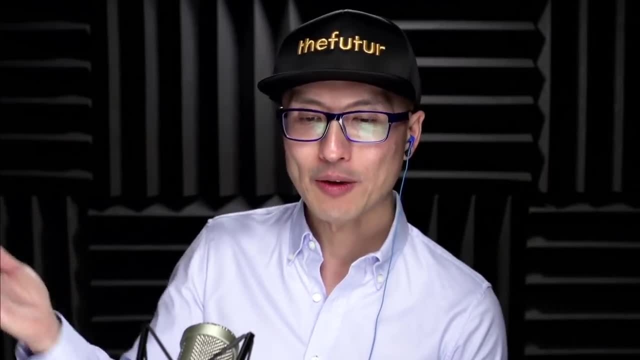 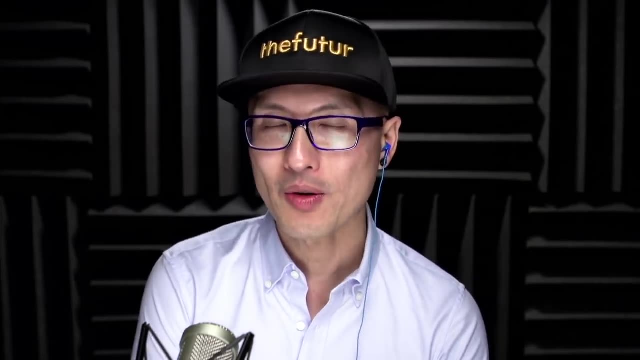 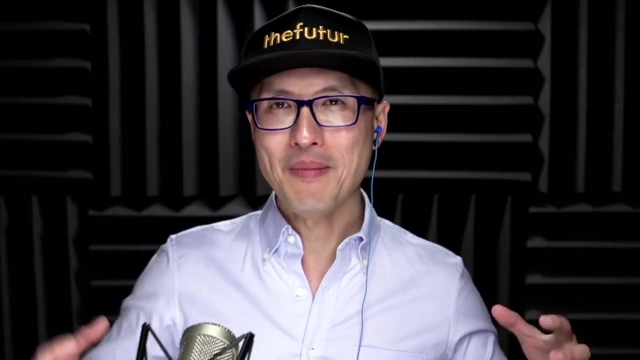 And therefore you shave off 14 years of learning down to six, And that's pretty awesome. So just don't be so impatient to say like I have to be there today, Because right now I suspect you guys, you young guns, are just trying to figure out who your creative self is in the making space. 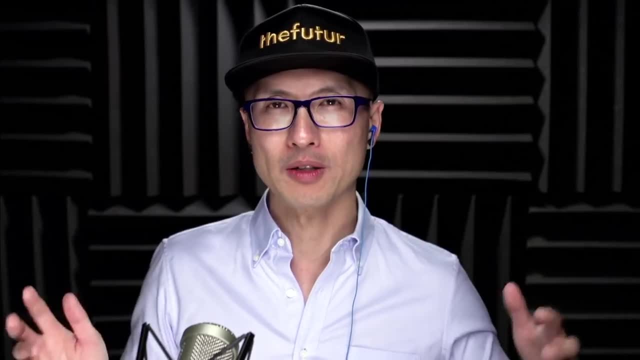 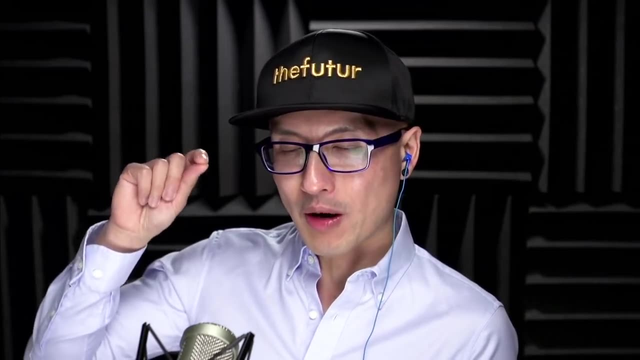 And there's nothing wrong with that. That's what I spent the first half of my career doing. Okay, So the thing is, it's kind of easier for you to look at from where you're at and look forward 20 years and say that's where I want to be. 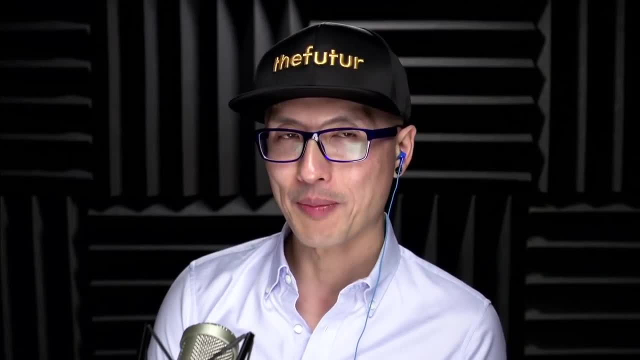 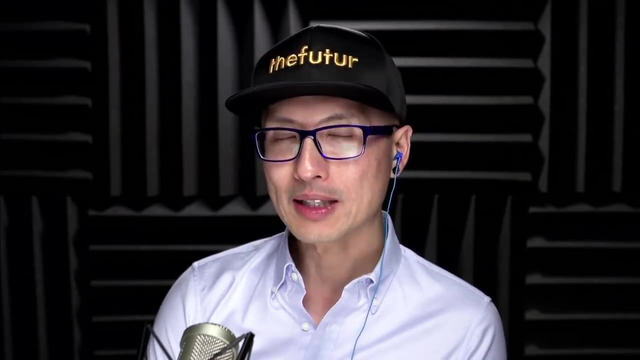 And then grow impatient trying to be there tomorrow. It's just not going to happen, And that's okay. If you come to that realization, you won't be so hard on yourself, And that's something that you need to kind of hold true. 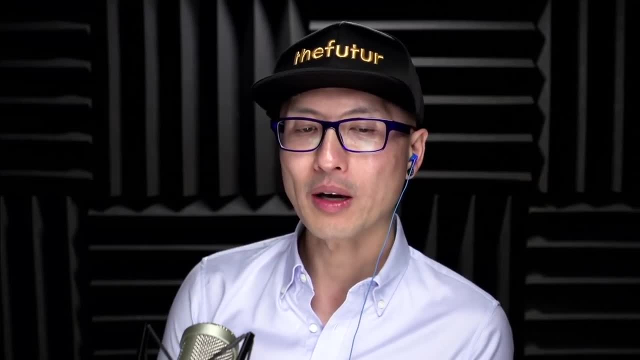 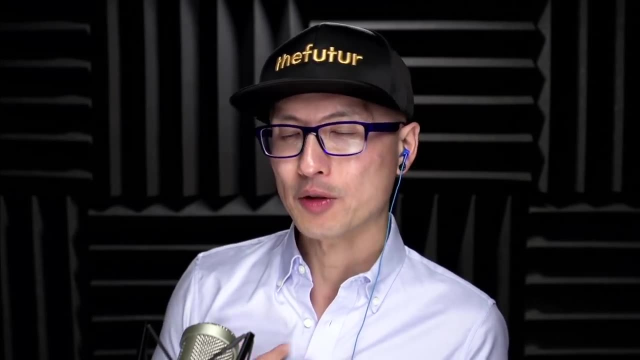 Otherwise you're going to become depressed, Like you want to work on branding systems. So there's still a lot you need to learn about branding. I only fully understood what branding meant and how to do it in the last five years. Prior to that, I thought I was doing branding and I was not at all. 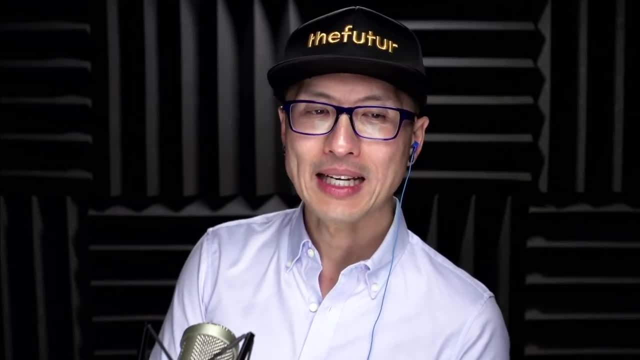 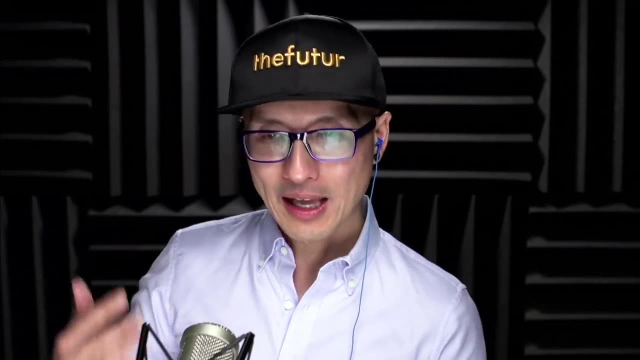 I was designing marks, I was creating identity systems, But I was not doing branding, Because branding is a lot more complicated than that. So why don't you master that? And as soon as you hit that pinnacle, set yourself a new goal. 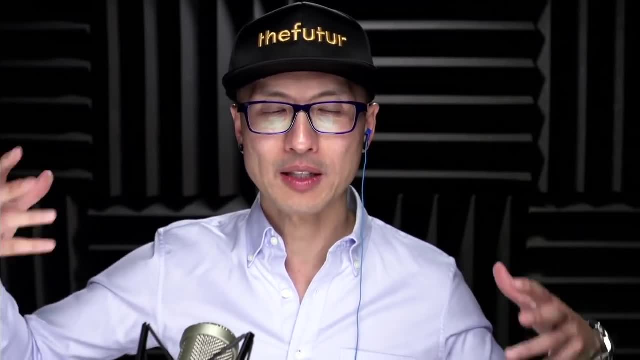 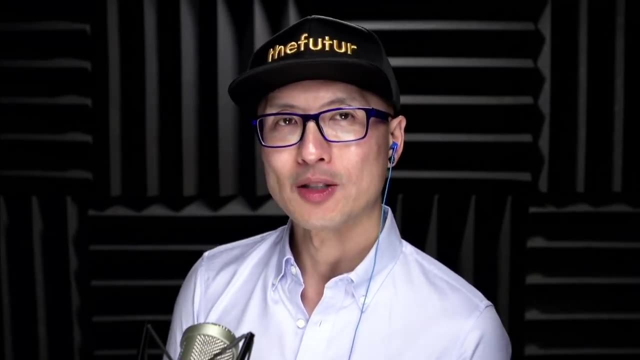 And just keep climbing, and keep climbing until you acquire all these different skill sets and points of view that you can help clients through most of the problems that they have. There's a good reason why I'm not standing in front of you as a 23-year-old. 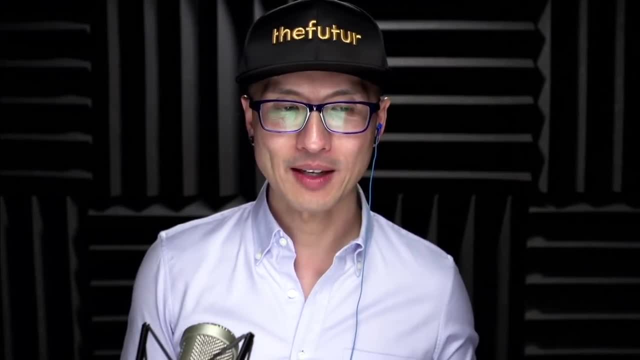 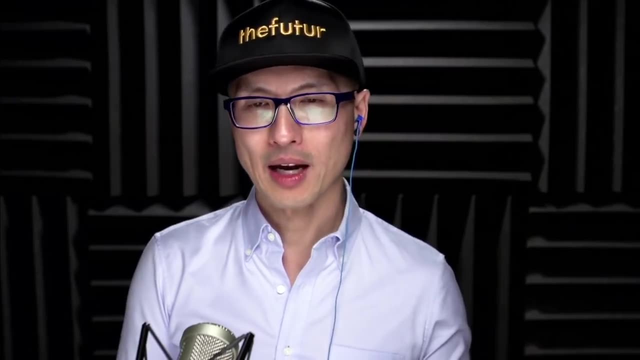 Because I wouldn't have those experiences to reflect on you right now. That makes sense, right? Yeah, it does, Alright. So guys, be a little patient here. Some of you are just coming out of high school, Some of you have some college and didn't even go to college. 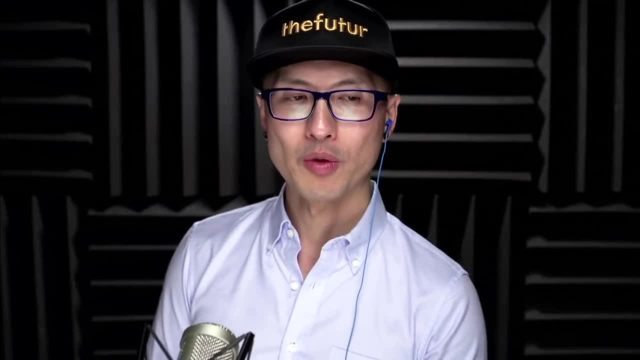 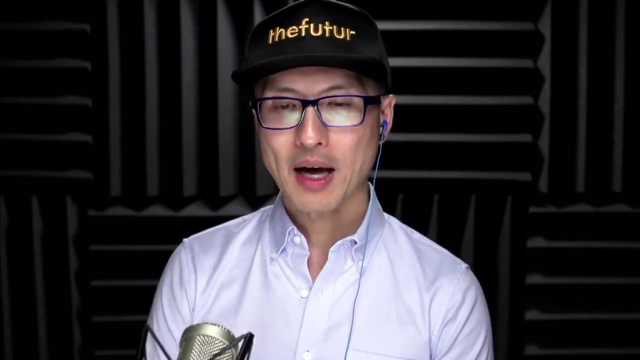 So just work on those skills, And I don't think Arun was being dismissive to Conor. Conor's done an excellent job of positioning himself, because everything on his Instagram seems to be about logo design, And so when somebody needs a logo, they're going to call him. 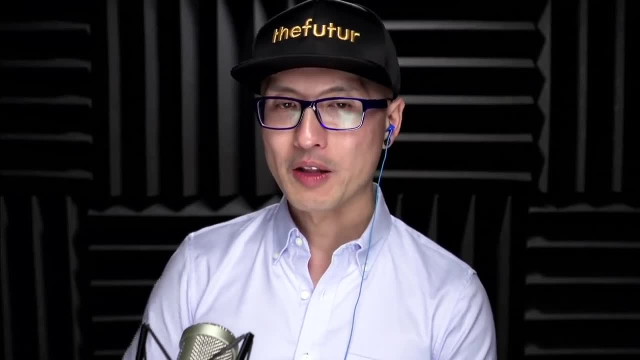 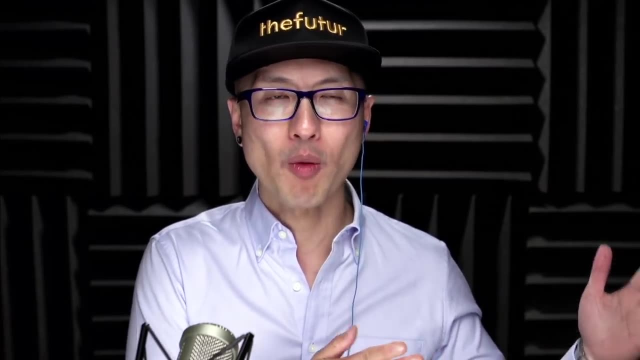 That's why he has work opportunities right now. But Conor, in the meantime, is working on developing his whole creative, his whole creative self And eventually he's going to flip the switch and migrate away from what he's known for into something he'd like to be known for. 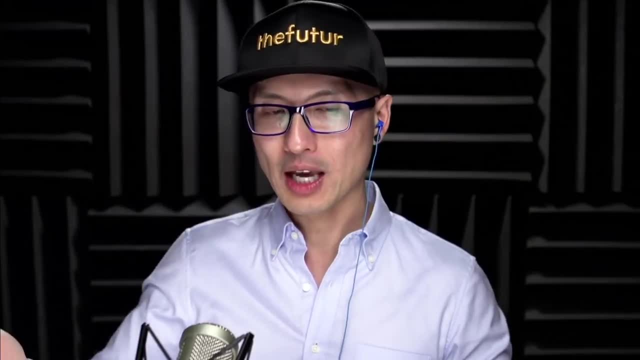 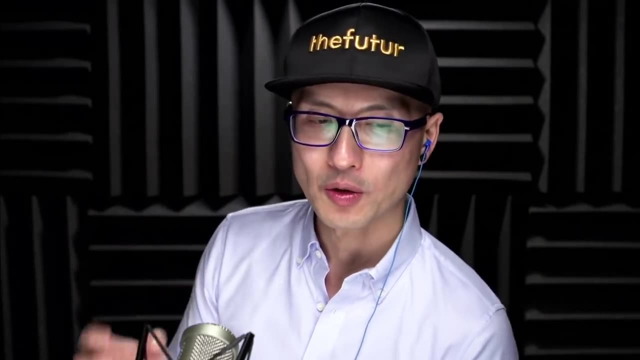 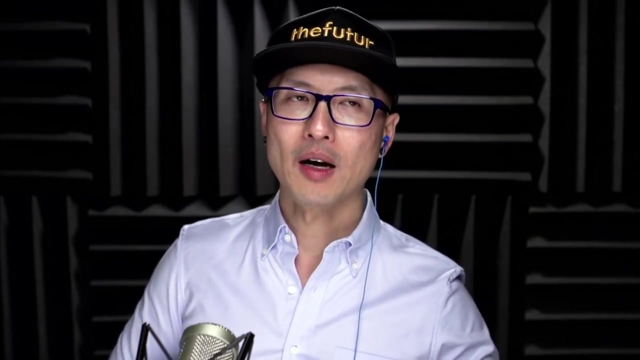 And so there's a transition period And you go through that and then you change again. Okay, Now let me just do like a fundamental, like meat and potatoes thing conversation. If you're watching this and you're thinking, what can I do, that's going to be valuable. so I don't get stuck in the maker space where it's not valuable and I'm going to be competing on Fiverr or Upwork or one of those marketplaces or 99designs. 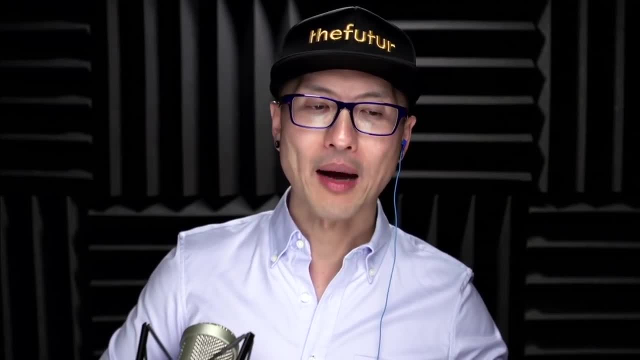 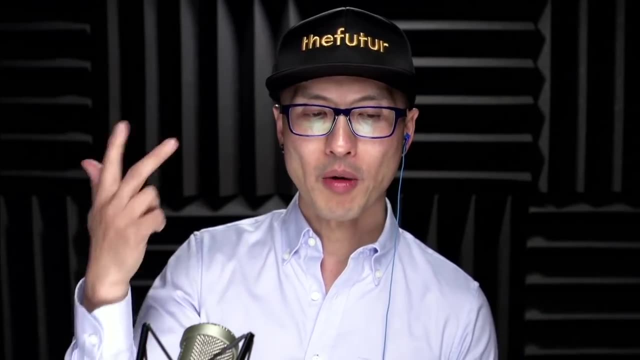 Well, let me tell you there's a couple of careers or career paths or jobs that you can have right now that are valuable to lots of people: User experience design, user interface design, social media marketing, slash content marketing. Those things are valuable. 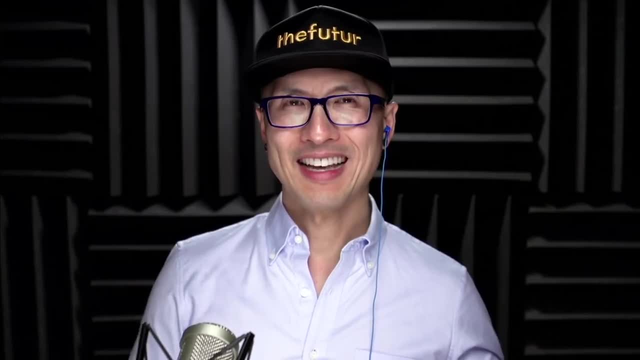 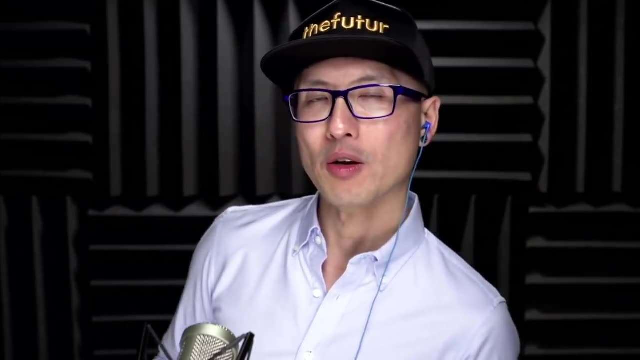 If you know how to build and create impactful websites, that's valuable, That's important to somebody. So those are the general four things I would focus in on. if you're still trying to figure out your career path, Is that cool, Yeah? 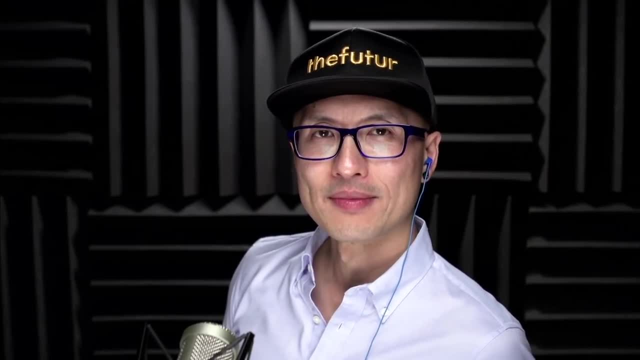 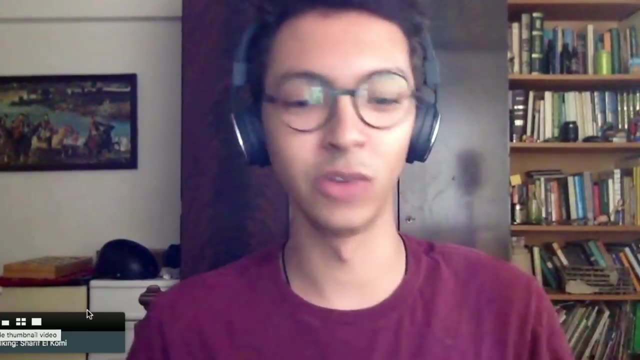 Chris, can I ask a question? Yeah, yeah, Earlier, you were saying that you wouldn't be standing in front of us as a 23-year-old. Yeah, Because you were still figuring it out and you've only figured branding out five years ago, and all that. 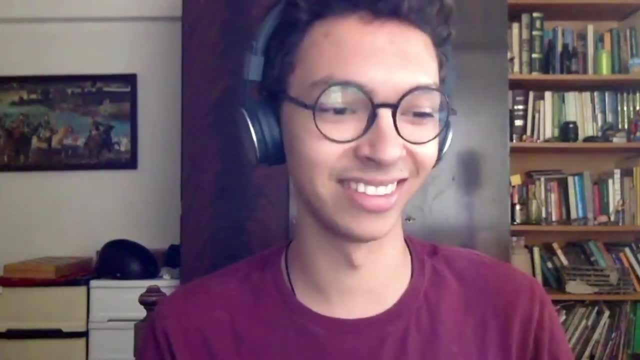 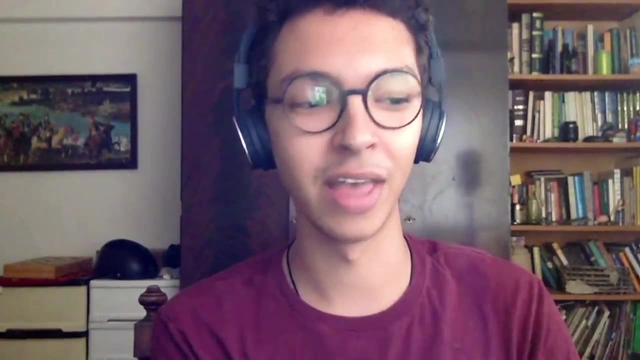 Yeah. So as a 23-year-old- and I just started my YouTube channel- I want to put content out there, And one of the things I struggle with is thinking that who wants to listen to a 23-year-old talk about branding or whatever I'm going to talk about? 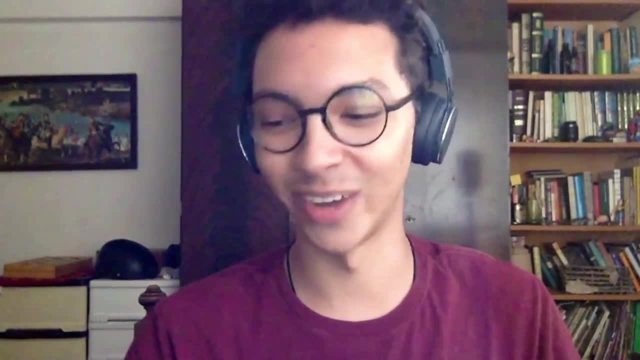 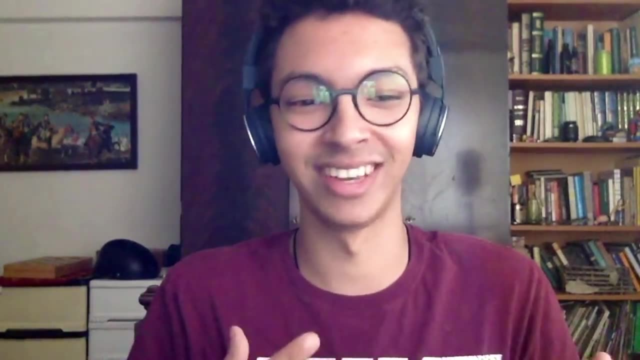 So how do I like? do people want to hear me? or am I still not a brand? Am I still not an expert, Like I always have this? I'm not. Who am I to go in front of people and tell them what to think or what to do? 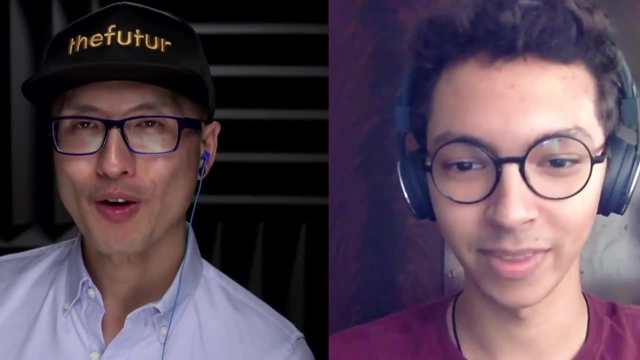 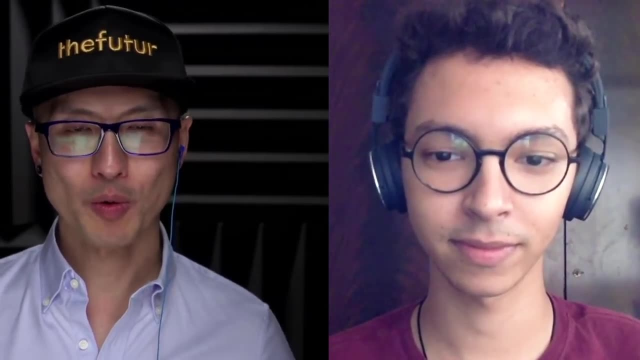 Well, you're not telling them what to think or what to do. You're just telling them your story from your perspective, And that's really important. Now, despite what I just said to you, that I'm not a 23-year-old standing in front of you giving you career or life advice, and we can accept that, that to be fine. 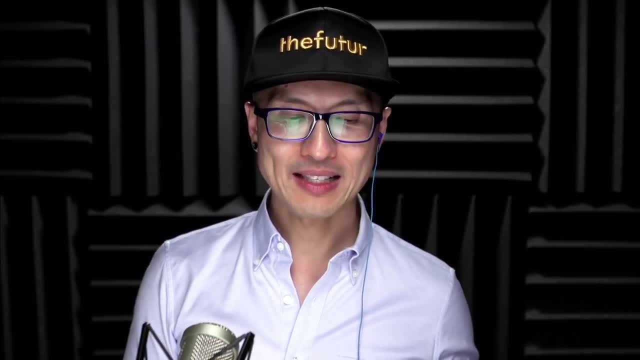 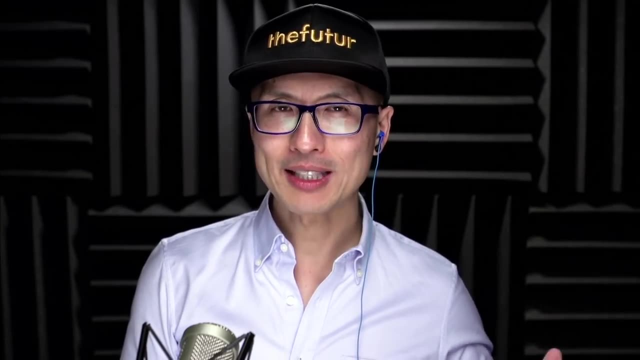 However: Demarcus, Brownlee, Logan, Paul, Casey, Neistat, Linus Tech Tips- Yeah, Linus Tech Tips. They all started when they were kids, I think Relatively young, And so the audience and the community grows up with them. 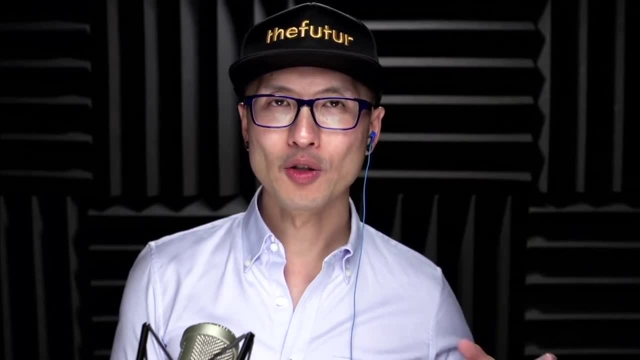 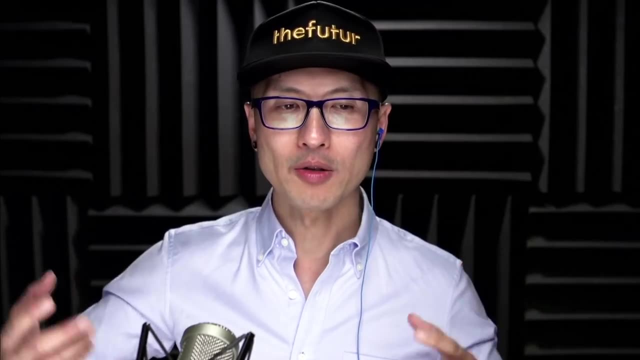 In fact, on YouTube I'm the anomaly, not the standard. YouTube is full of young people sharing their story, their life experience, So there's value in just learning along with you and traveling along your side as you go along your journey. 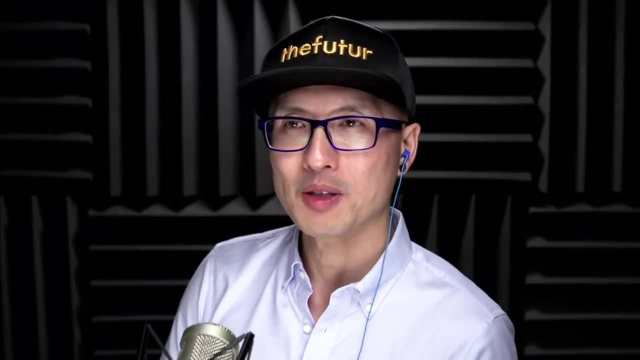 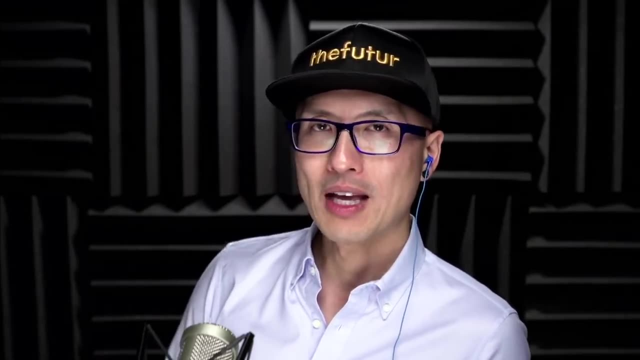 And that's valuable to lots of people And that's why they have so many subscribers, because somewhere in the universe, because they're young people watching YouTube, they're going to say: I relate to that person, I relate to Sharif, I'm also from a developing country. 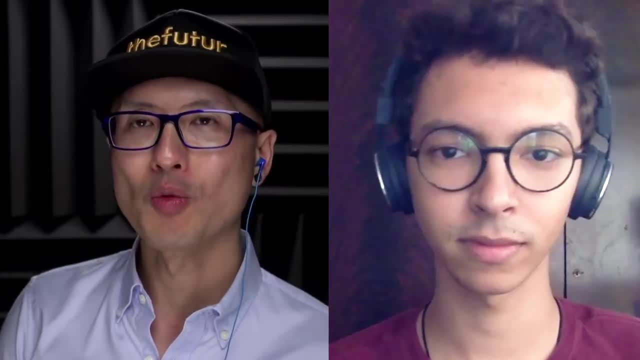 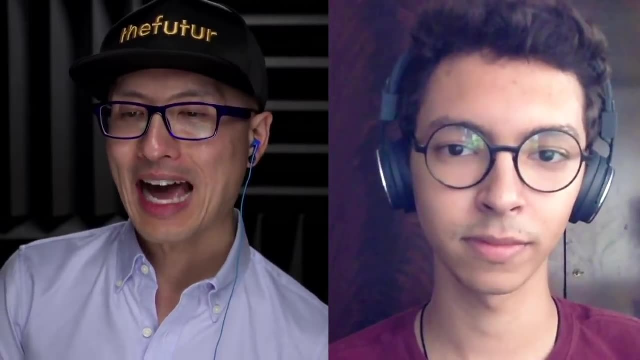 And I'm also struggling with self-confidence. So what you want to do is not to try and stand there and say: I'm the expert, I figured this stuff out, This is what you need to do, But to say like I'm still figuring it out. 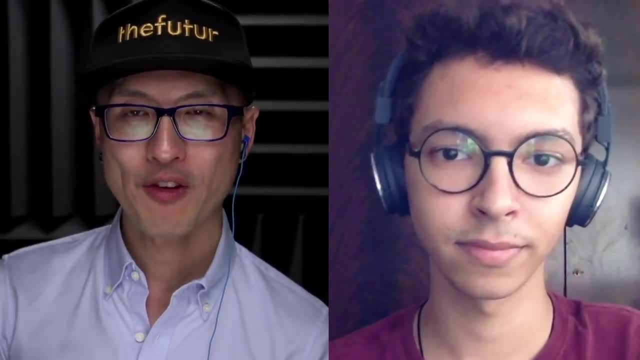 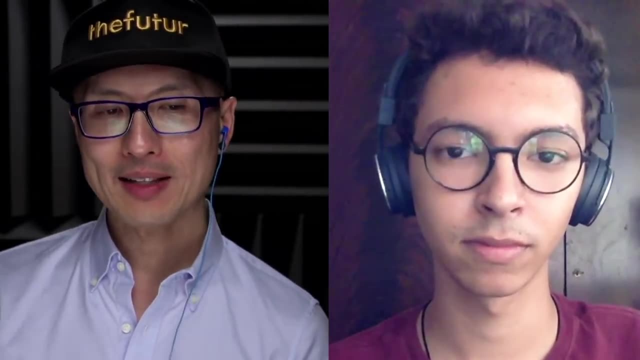 I'm not sure what it is I'm supposed to be doing, but here's what I figured out so far. If this helps you, keep watching, Stay along with me, Come along the ride And we'll grow together, And that's actually more valuable than just saying: here I am. 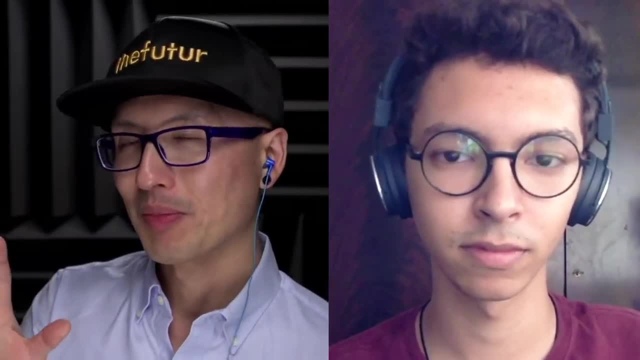 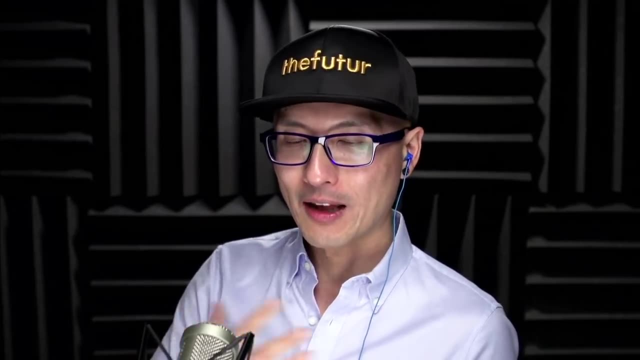 Here's what I've done. So you see, here's the interesting part. You guys are asking me lots of questions about how did I make that mental switch? How did I start to think to myself: I'm good, I love myself? 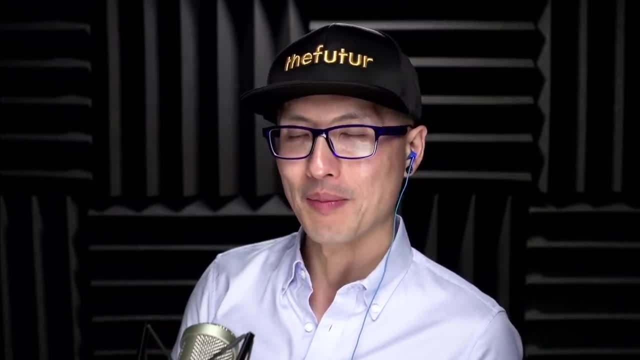 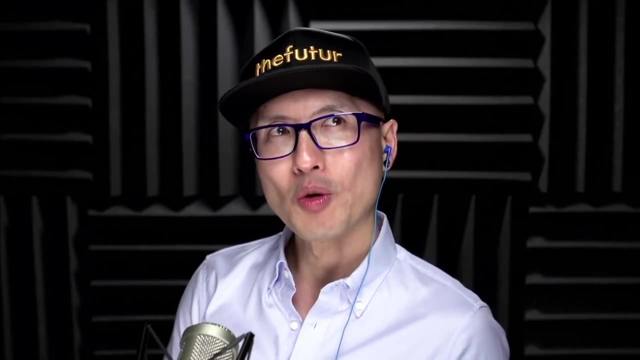 That I'm great. Well, I can't share that experience with you in real time because it didn't happen. now I have to look into the past and I have to recreate in my mind like what were those moments. But imagine if you were watching this channel. 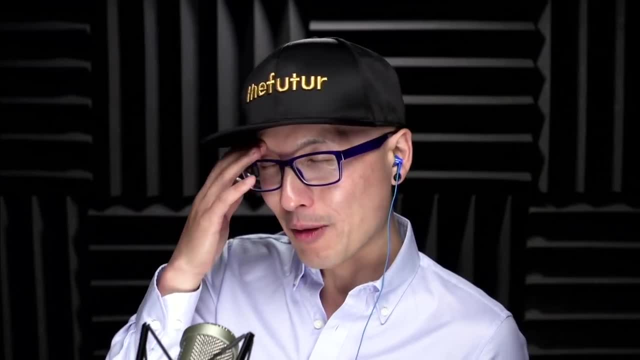 One day I'm coming to you. I'm like crying my eyes out. I'm like, oh my God, Today was a really bad day. Here's what happened. Right, I'm feeling, I'm happy. I'm having suicidal thoughts right now. you guys, 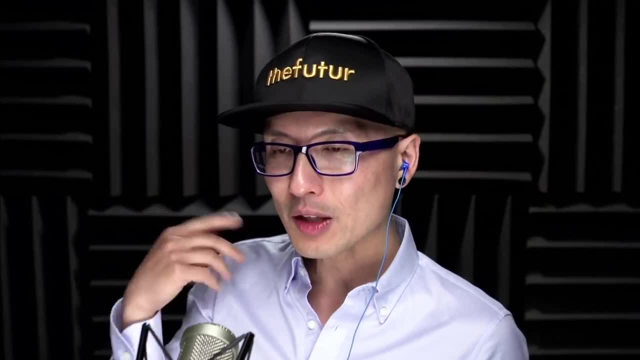 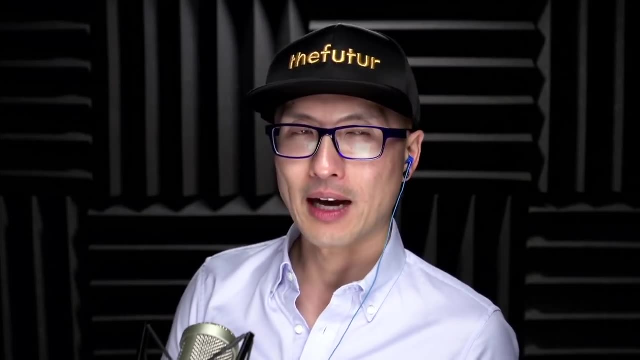 And then all of a sudden, the next day, two days later, I come back and say: look, I went down this dark path. I wasn't sure if I was going to make another video, But here I am. I figured it out. 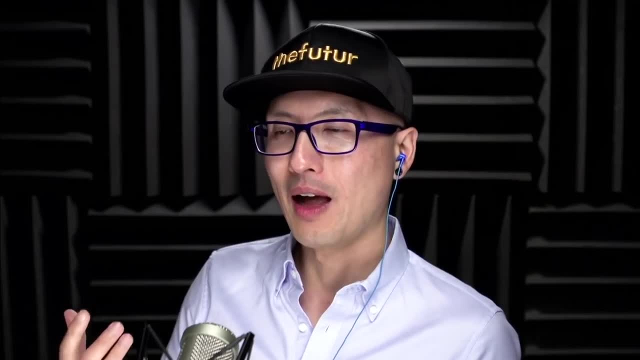 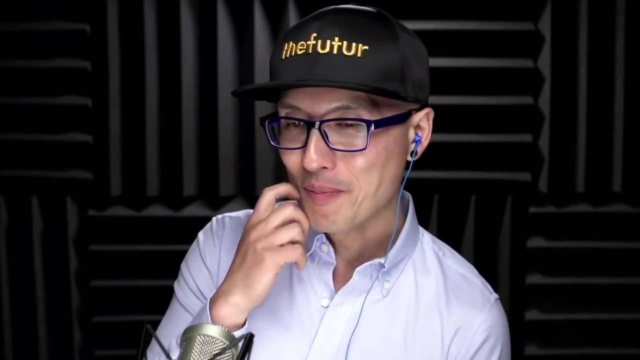 This is what I want for my life. Stick around with me, guys. You're going to see things change And you see that happening in real time. It's like a real time drama that's unfolding in front of your eyes. I'm pretty sure that would have a lot more views than the channel that we have right now. 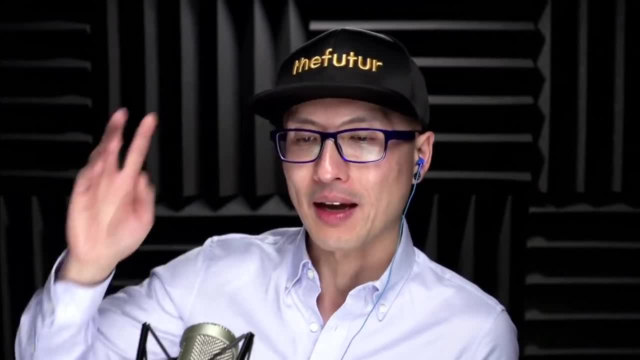 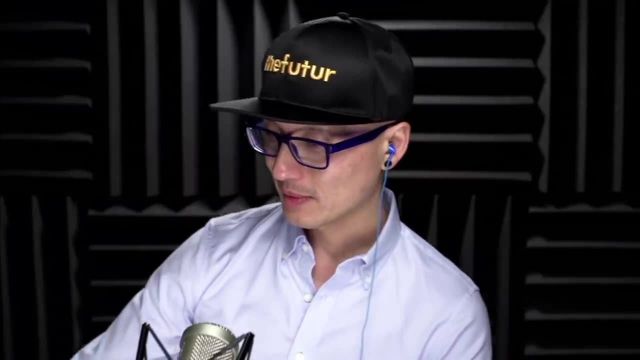 You understand that For all you, young people, youngish people, young in mindset, don't be afraid to produce a video. Just be honest and transparent, because that's what people want from you. Okay, And we talk about that a lot. 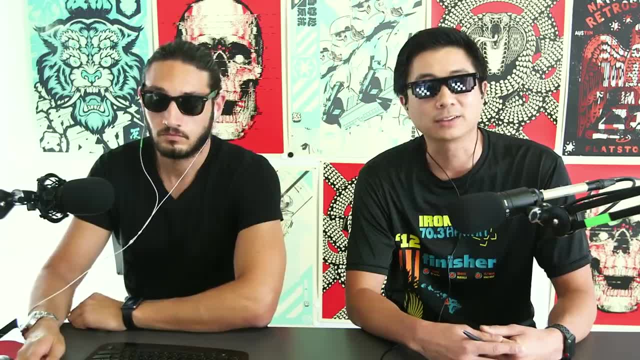 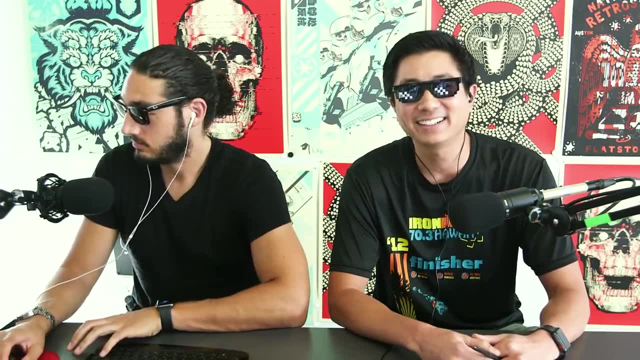 Vulnerability really makes you relatable with people. Yeah, That's why I'm not that. That's why I'm not so relatable, unfortunately, Because you're a robot. Yeah, So you know, when I was in the Philippines, somebody had asked this question like: what's your weakness? 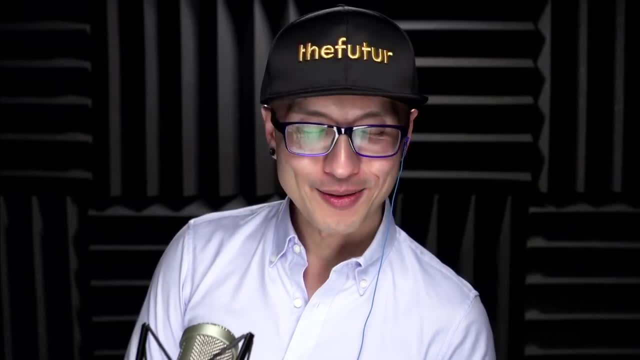 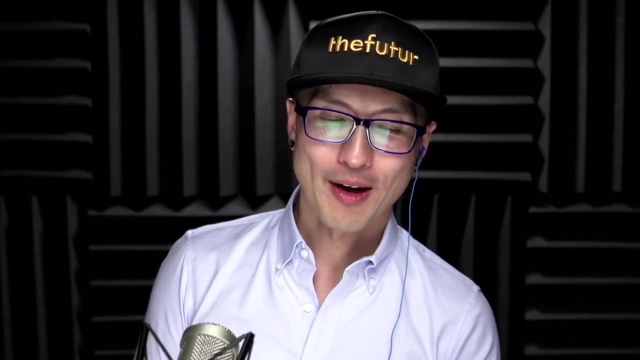 What are you bad at? And I said: oh guys, you have to ask that dark question. here We're trying to celebrate positivity and have the right mindset. I said: I don't know Why don't you ask my wife? 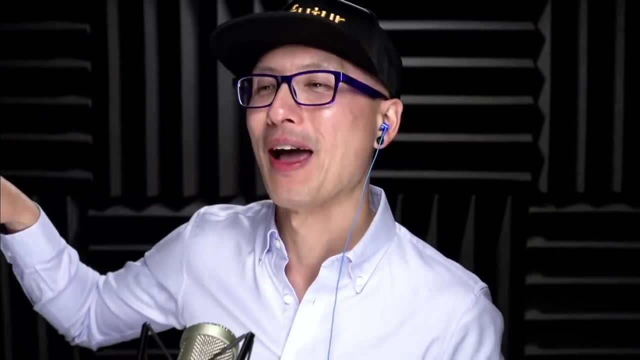 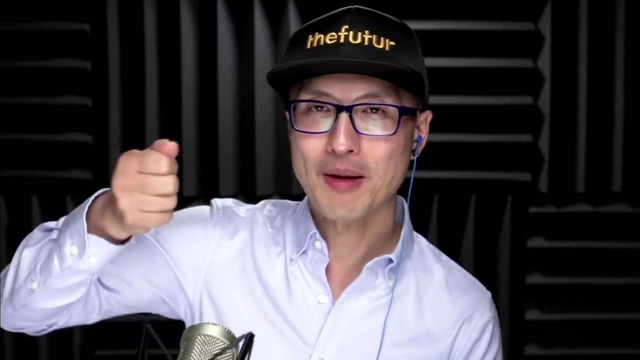 And so the camera and the spotlight is like looking in the audience for my wife And I can see her ducking behind people like do not pick me. And then I said the best person to ask is my wife. So eventually the microphone gets passed over to her. 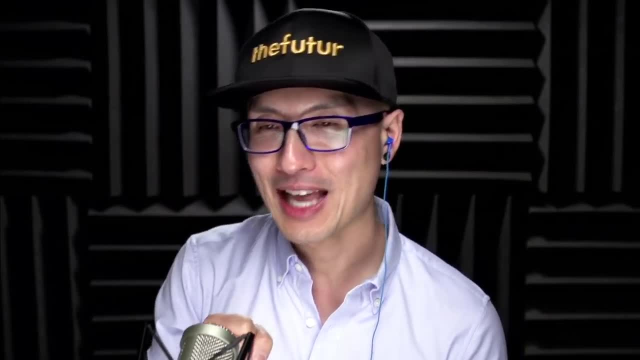 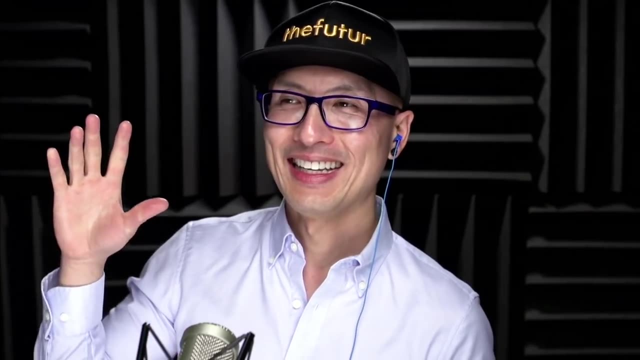 She grabs it And first she says he doesn't have any. And then everybody like laughs and cheers- I'm like honey, don't say that. And she then corrects herself. She says he believes he doesn't have any. 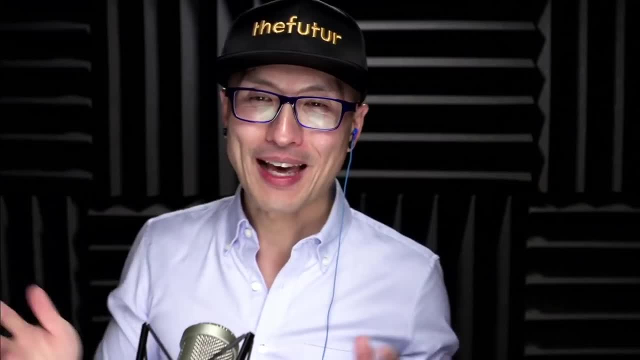 He believes he doesn't have any. Then everybody erupts with laughter. And maybe that is my weakness. I don't believe I have weakness, I don't know. That could be it. You can't recognize your own weaknesses. That's your weakness. 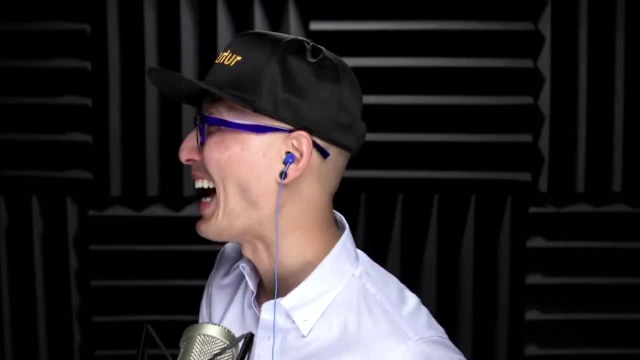 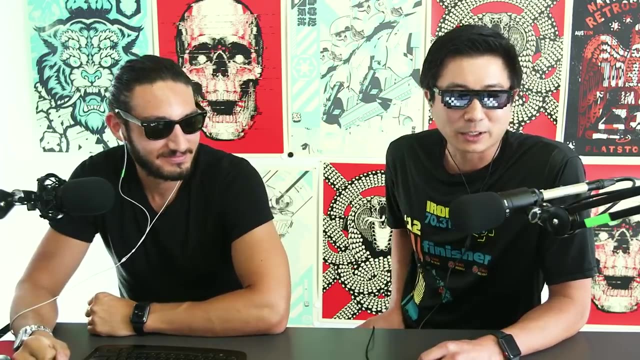 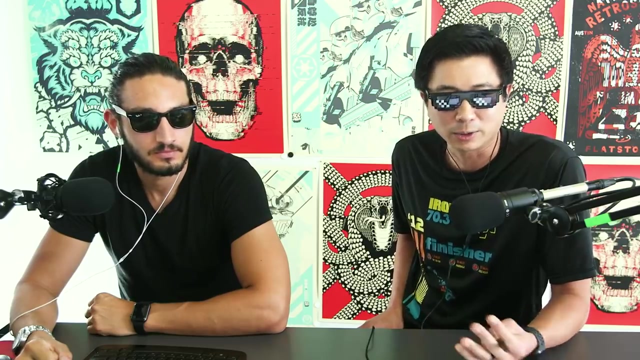 I have none Either way. There was a good comment that came up here from Cesar And he was just talking about sometimes people look for younger folks to get their input, especially with a lot of new media, And he was referring specifically to social media. 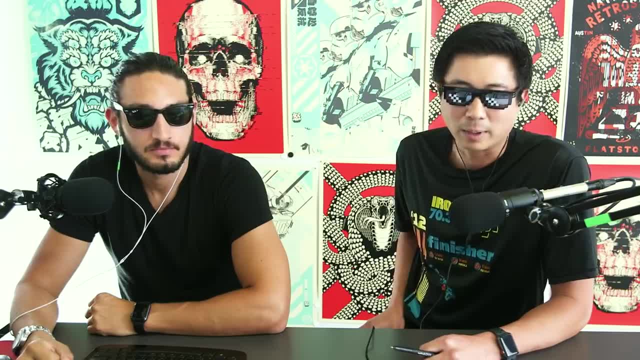 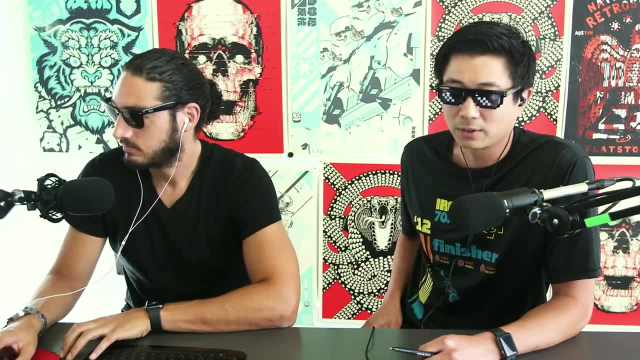 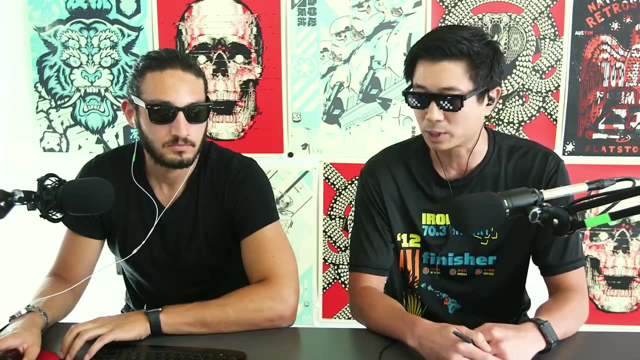 So, Sharif, you're talking about how maybe people perceive you as this young person that doesn't know much and you're not as experienced, But people look to young folks for stuff that old folks don't need. So I think that might be another approach to things, where you could feel like you might be more of a specialist than someone else. 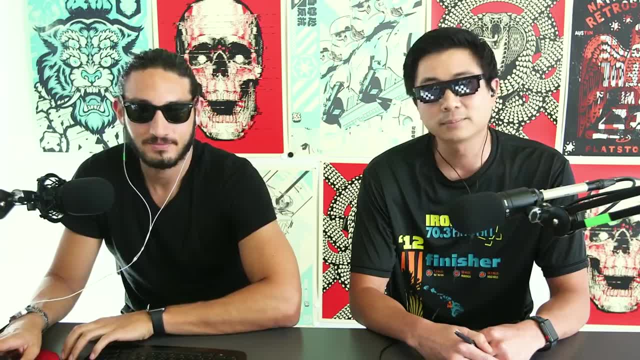 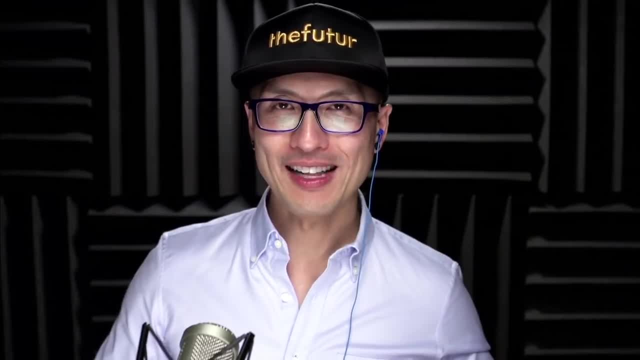 Because you're young and you know what's cool- These young, dumb and broke high school kids, as the song goes. Now you know what Young people should be fearless. They should just throw caution to the wind and be willing to try anything and everything because they don't have much to lose. 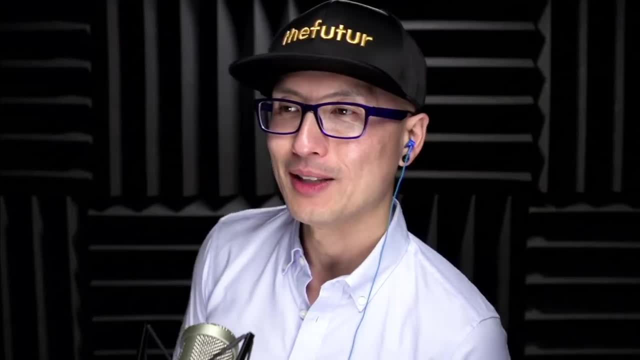 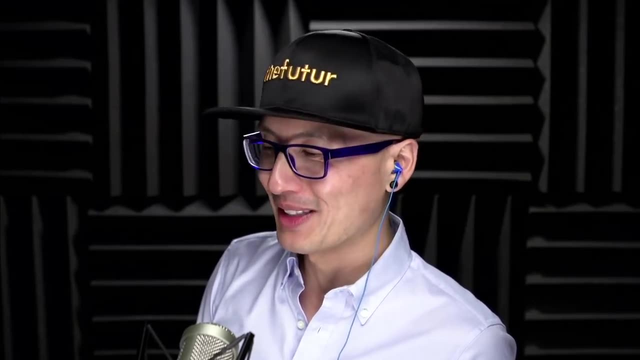 And that's the fantastic part about being young: You can walk into a gym, get punched in the face and you can bounce right back up. You can go snowboarding, break your ankle and just bounce right back up. When you get old, you break your hip. it's game over.